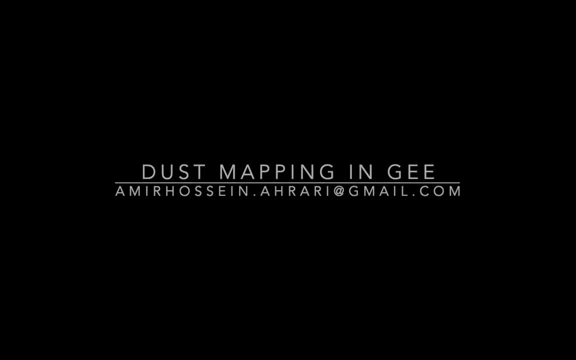 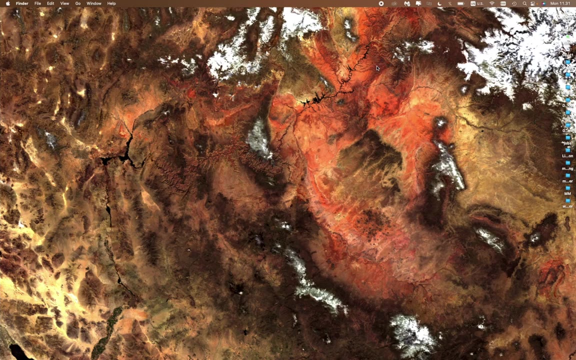 Hello everyone, Welcome to this video. My name is Amir Sinafari. I'm a Google Earth Engine expert. In this tutorial, I'm going to show you how to do dust mapping in the Earth Engine platform and remote sensing data. Let's go to the code editor environment. 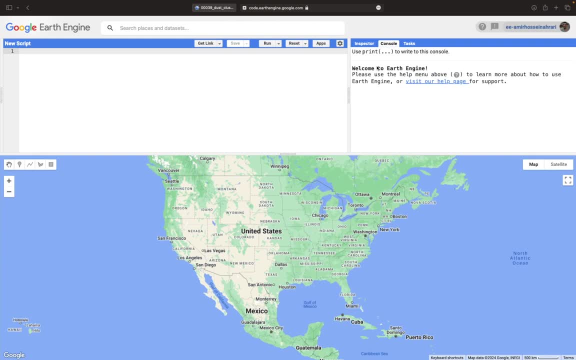 Unlike the previous studies, now we don't like to set the region of the interest, because we want to do the time series analysis and clustering mapping in this tutorial only in the global scale and no need to select a specific region as a study area. So in the 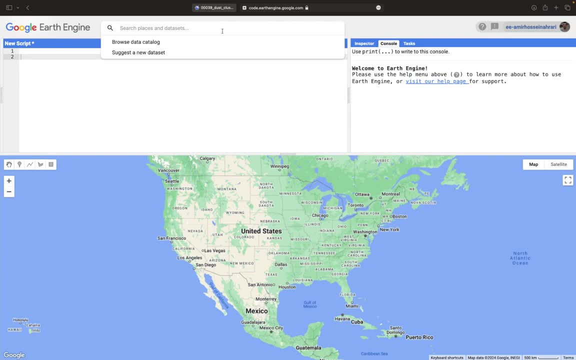 first step, you need to find your desired data or target data through the search places and data set. If you search through Mera2, you will see that all Mera2 products are available here. As you can see, one of the Mera2 products is RSL Diagnostic helping. 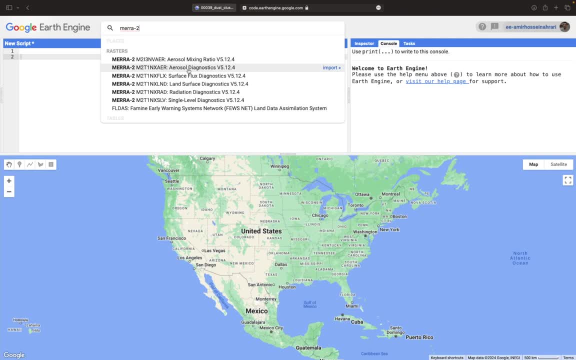 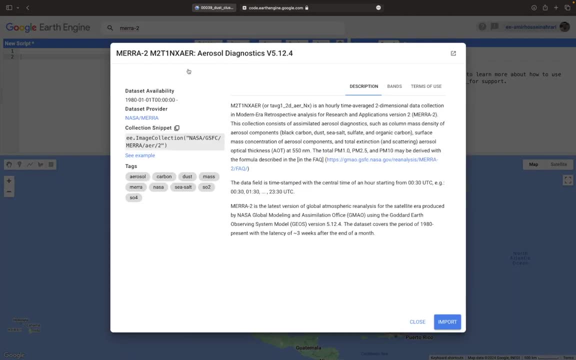 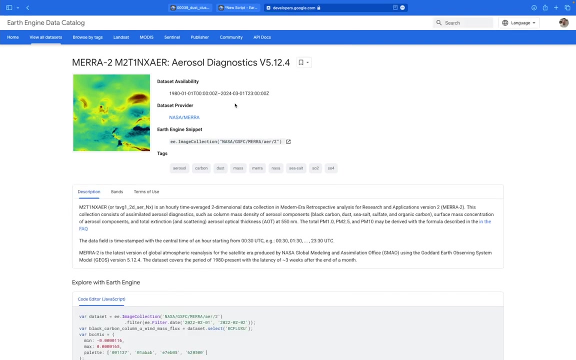 us to identify RSL characteristics in global scale with 50,000 meter spatial resolution. Go to the data description here and then you can check all the information related to this product. This product is available since 1980 to 2024.. Let's go to the data description. 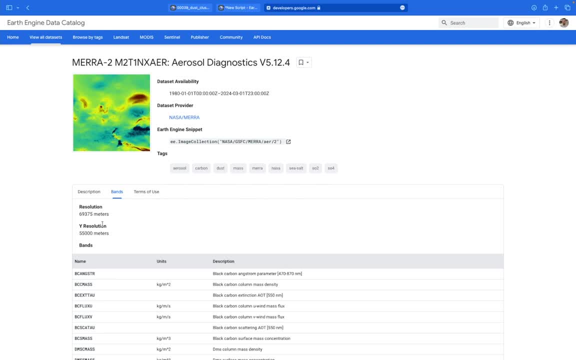 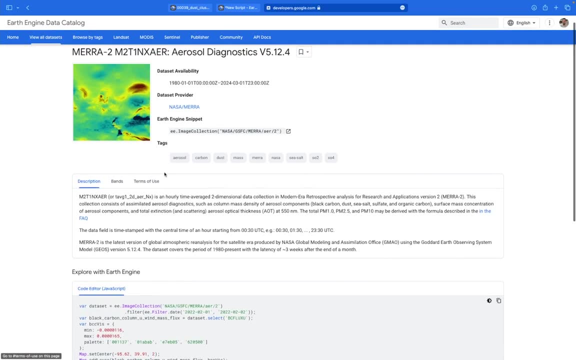 This product is available since 1980 to 2024, with 50 meter roughly 50 kilometer spatial resolution and hourly temporal resolution, The hourly time average or temporal resolution, helping us to monitor the dust variations accurately. So and 50 kilometer spatial resolution. 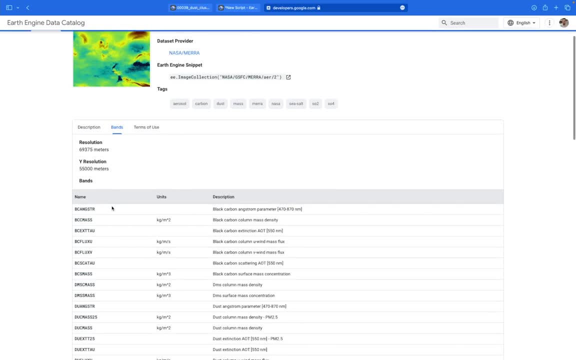 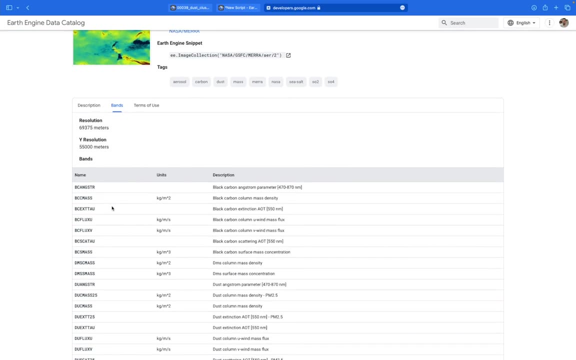 is too coarse, I know, but this product is specifically used for the global scale. Most of the time our studies cover the global scale, but this product is specifically used for local study study or major study or cinematic districts or historic places in the global scale. We usually focus on the local studied area, but especially for the 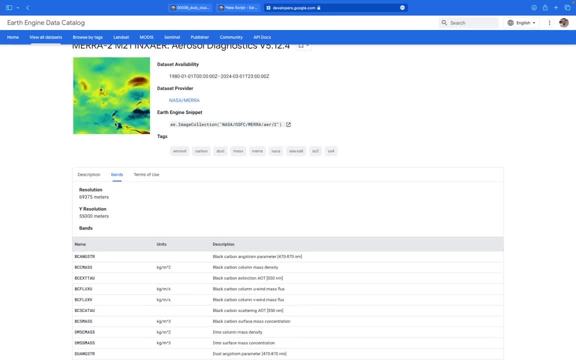 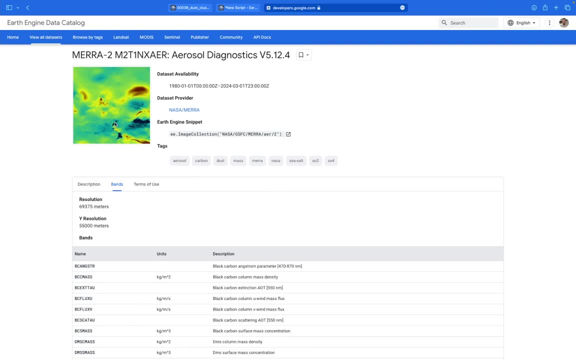 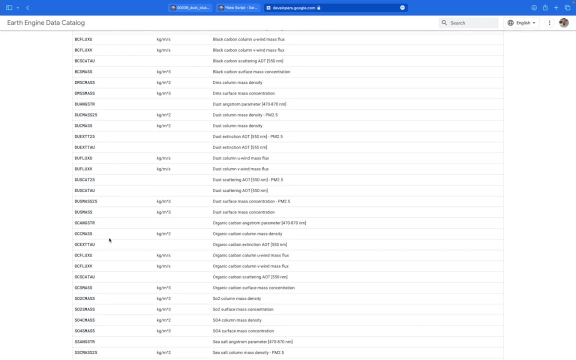 dust studies, because dust is a kind of catastrophe that is happening on a very large scale and various spatially and temporaly, from one hour to another hour. As you can see, various bands available here and all of them covering different characteristic of the dust. For example, one 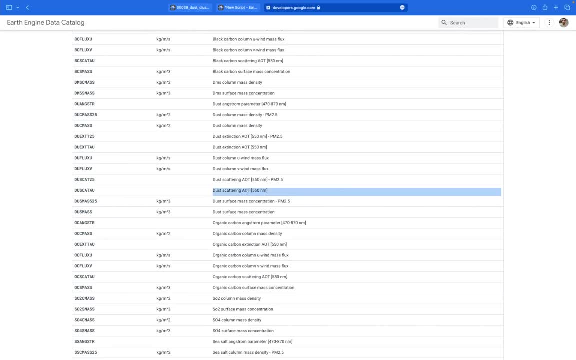 of the most famous dust here is surface tact, which is newly used in the areas near employer's data is our soloptical thickness or our soloptical dips in 500 nanometer wavelengths. that's highly useful for the dust monitoring and global studies. so 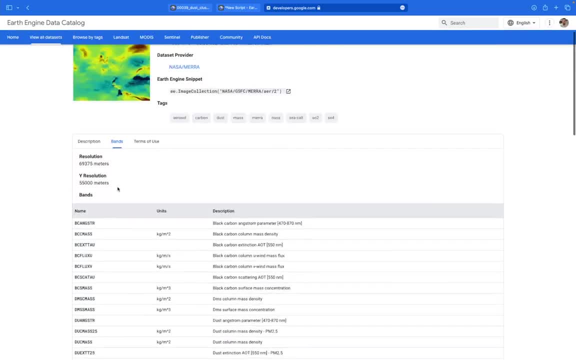 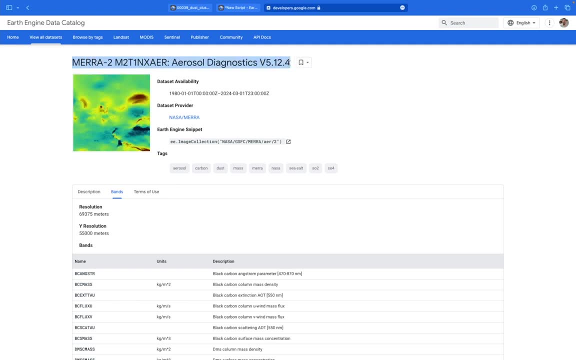 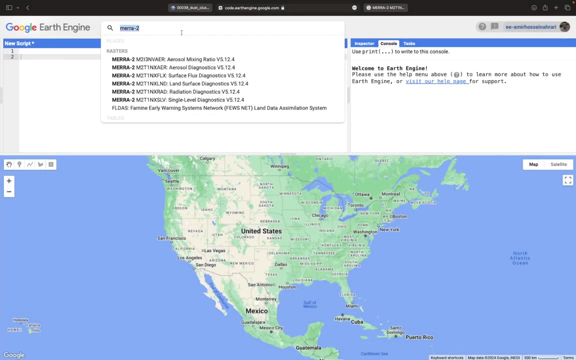 with the spatial resolution it has. so now, in order to use this product into the code editor, just copy the name of the product and paste it into the search places and data set. here in search places and data set, paste the data information as you can see, and here you will see that the mirror to product. 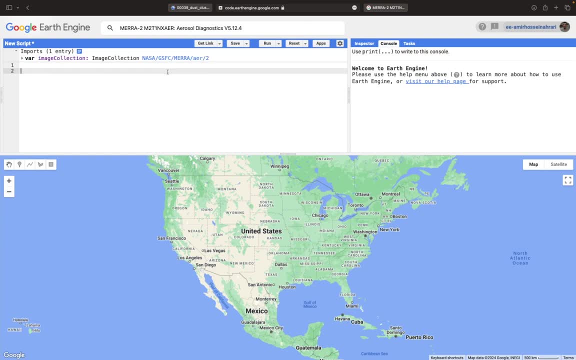 also diagnostic is available, imported into the code as an image collection and then make a variable for a new variable as a OT. our soloptical thickness equals to the image collection imported and now, as this data is hourly, meaning that for each day we will have 24 a OT. 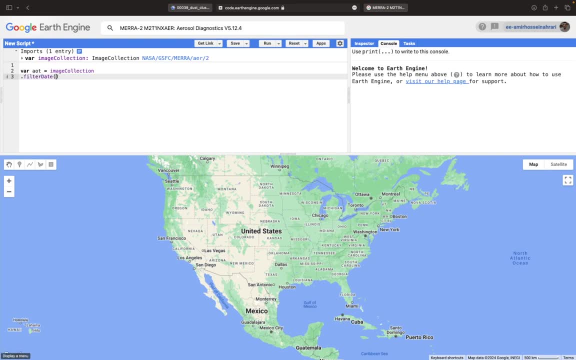 image. so, for example, throw the filter date- you can check it- the time start, for example, since 2010, the first January of 2010 to the second January of to the second of January, like this, and then print the a OT in the right panel. you will see that only for one day. 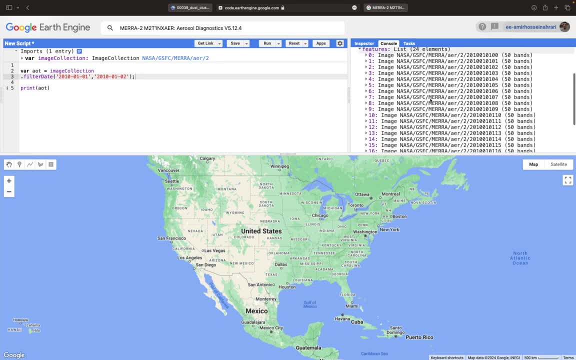 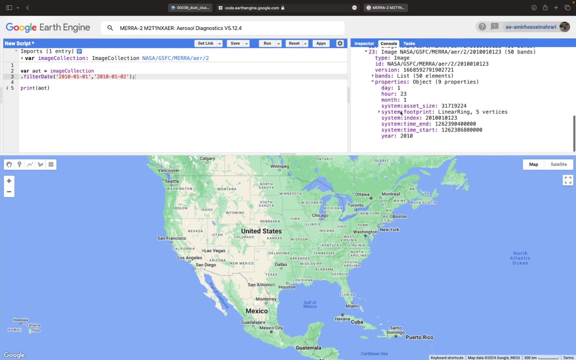 we have 24 elements. 24 elements starting from 0 am to 23 pm. as you can see, this data available and also in the properties: the hour, the amount and the day, also separated. now I'm gonna show you a technique to. 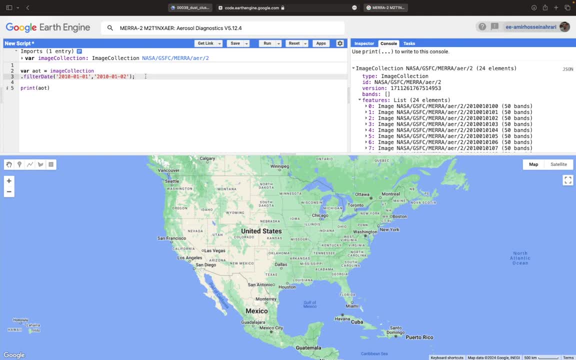 help you to select the data according to a specific hour, or according to a specific Mount or a specific date, using calendar range. for example, let me set a new temporal range from 2010 to 2011. so here, for example, we want to do the dust. 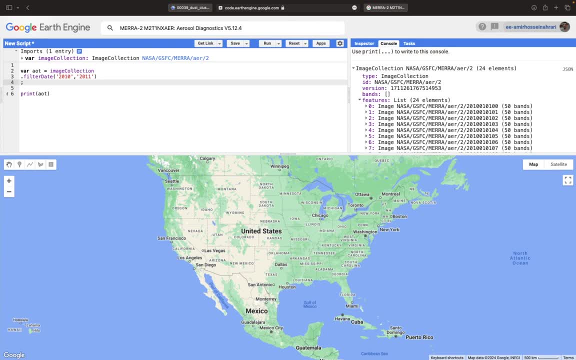 monitoring, just only based on the data collected around, for example, the 12 pm. so and then make a new filter to do this. make a new filter and using calendar range- earth enginefiltercalendarange- we will be able to filter our data based on different temporal filters. so in the left panel, go to the dock to understand which kind of filters available. 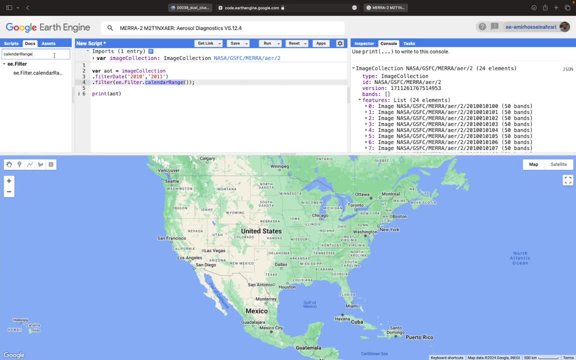 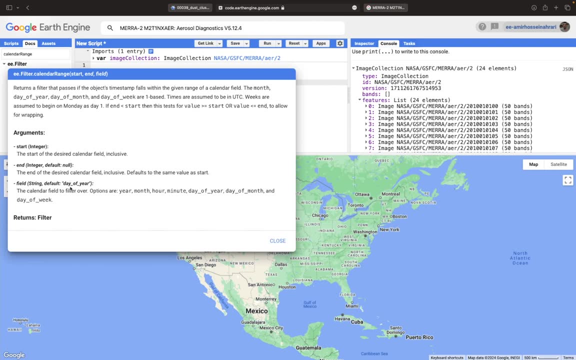 through the calendar range. just copy and paste the calendar range inside and, as you can see, here we have the calendar range with different field of with different fields. you can filter your data according to a specific year or amount or hour or minutes or day of year or day of month or day of week. it's very, very helpful for the high temporal resolution data. 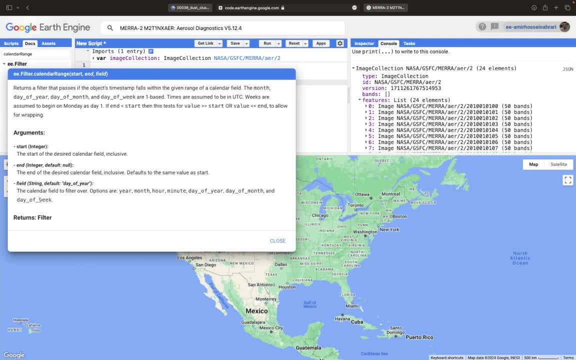 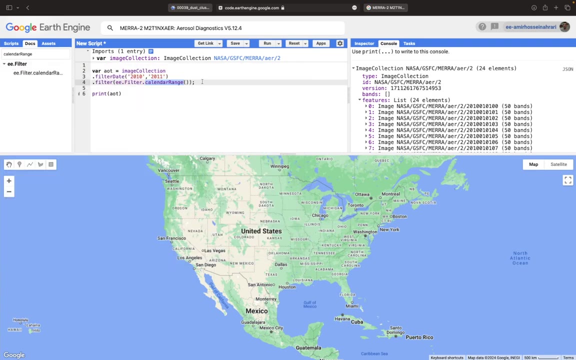 you are working. now i have a hourly data and also using this filter, i can only select a specific or a single hour to for the analysis in the next step. so imagine that now, through the calendar range, i want to select all data from each day. i want to keep the data for uh, 12 pm, so 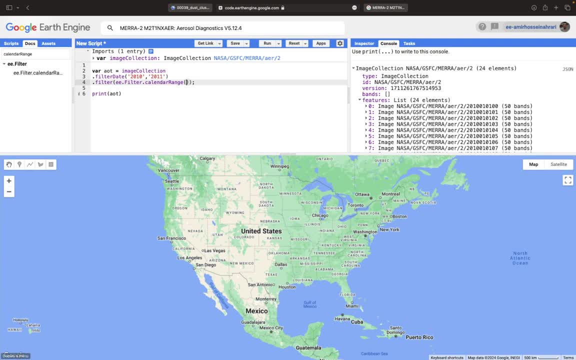 enginecalendarange here and some arguments available: the start, end and field, as i'm gonna filter the data based on hour. the field should be hour and i want to get the data for 12.. like this, run the code and finally, we will have a third: 365 elements available here, as you can see. 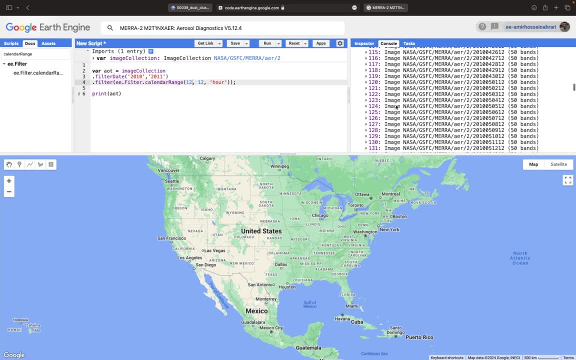 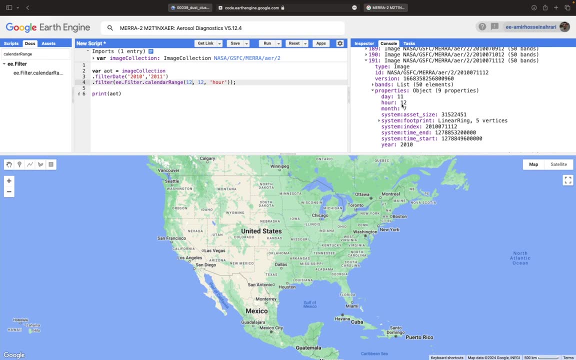 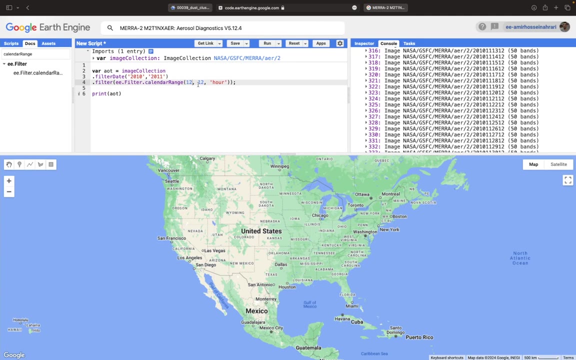 all of them are for our 12.. as you can see, randomly, when you check them, you will see all of them available for our 12.. so and the calendar range helping us to filter our data based on different characteristics or based on different temporal characteristics regarding to the temporal. 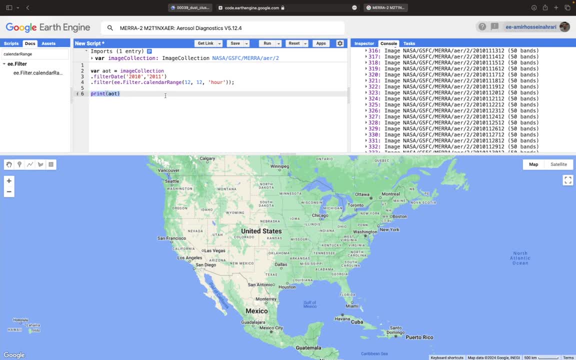 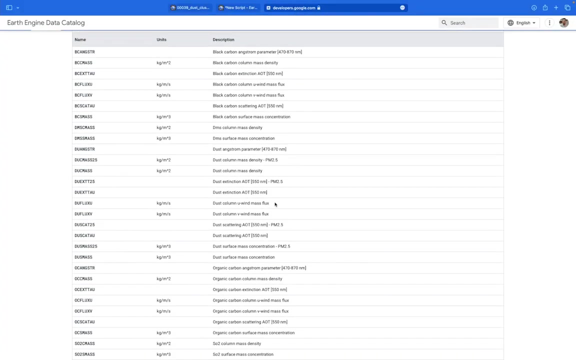 resolution we have. so in the next step i'm gonna show you how to visualize the global aot map, but before that you can see for each date 50 bands available. if you go to the bands you can see 50 parameters or factors available regarding to the dust condition through the band information and description. here you can find your desired or 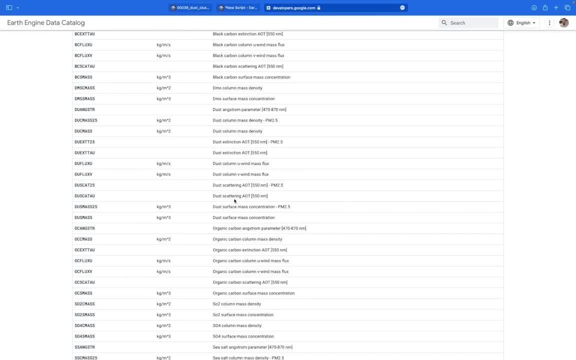 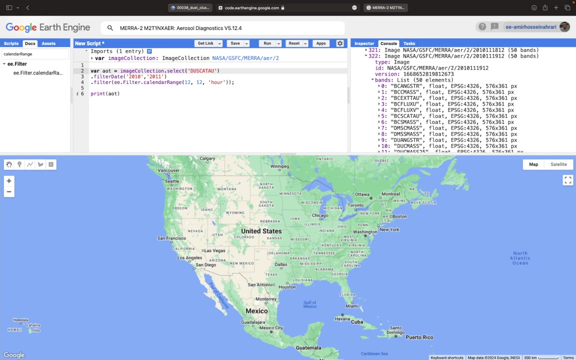 target band. as i as i am gonna working on dust scattering or aot, my target band will be this: copy the name of target band and throw the dot. select will be able to select the only dust scattering or aot according to the 500 nanometer wavelengths. run the code again in the right panel. you will see a new collection. 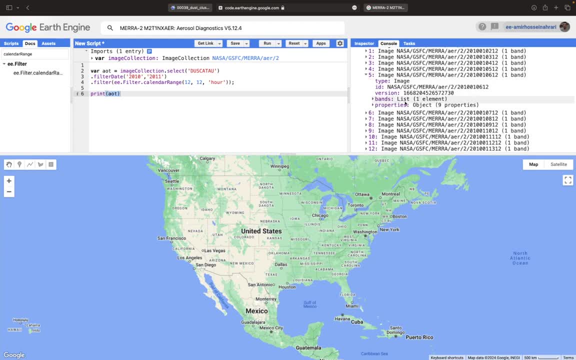 of elements here and you can see that we have 365 elements under each, with one single band, that referring to the aot for our 12.. so in the next step we need to do visualization process. to visualize 365 image, we need to stack all the images, all the elements, into a single file. 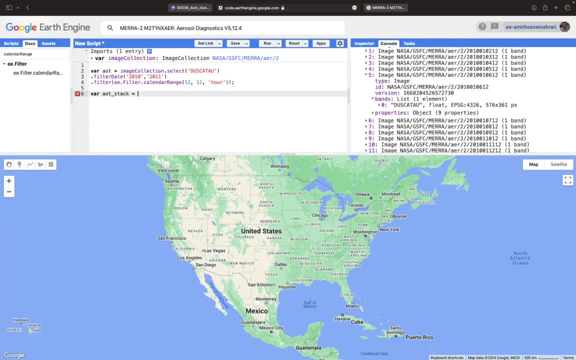 make a new variable. aot stack equals to get all images under aot variable and throw those two bands, stack them all into a single file, into a single jot files with a 365 bands in which each band showing the hours of condition for each date. so now, if i print a ot stack, you will see a new. 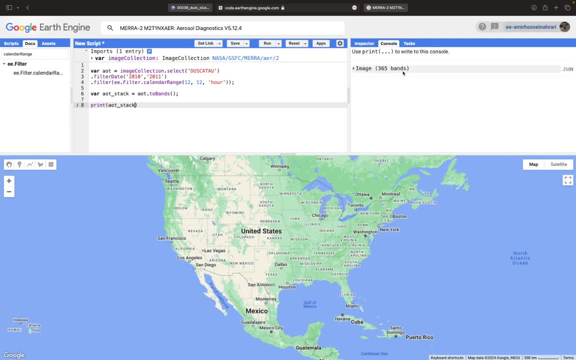 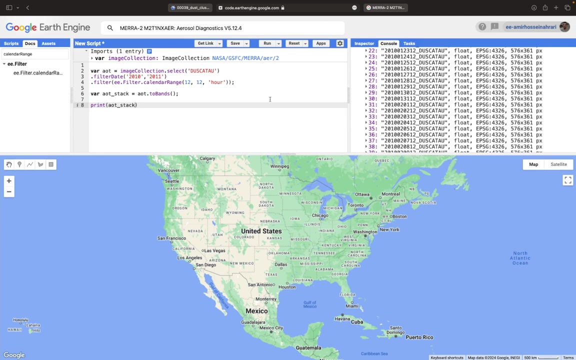 image is created with 365 bands, 365 bands available, one file with 365 bands and each of and also each band showing the dust condition for a for a single date. so then, through the mapadd layer, you will be able to visualize a ot, a stack, no need to clip it based on a ot stack. 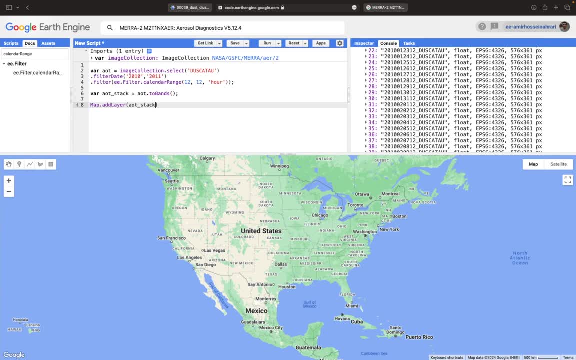 the region because we want to see the result for the global scale. We can do it for the coarse spatial resolution data because they have no framing structure and low spatial resolution helping us to do such kind of visualization process in the Earth Engine platform easily. So leave the visualization parameters empty because we don't have only one band into. 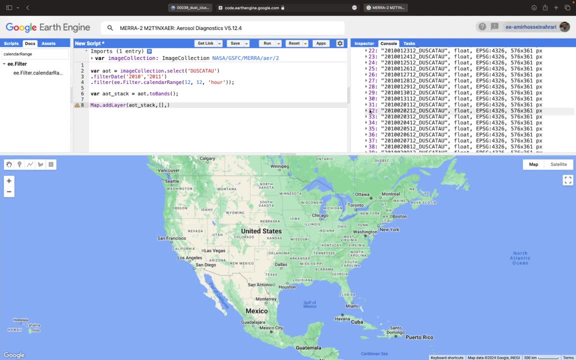 a stack vault, multiple bands available, and as multiple bands available, we can't set a specific visualization palette or something like that. So then the layer name is AOTStack and then use the false- false, helping us to avoid automatic visualization that highly reduces the speed of processing in the Earth Engine. 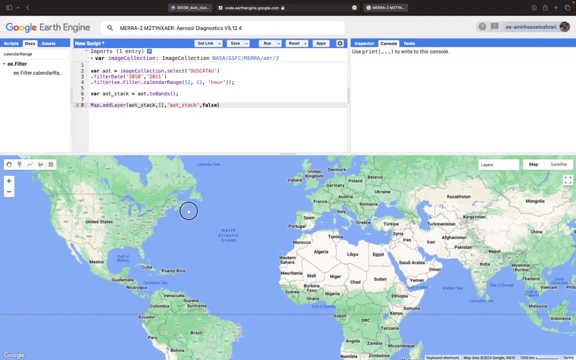 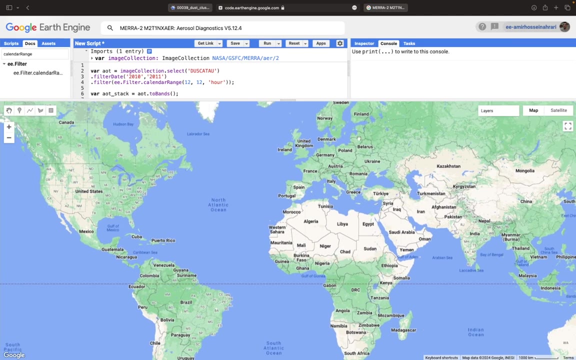 Run the code and change your view, Using tools available here or using mouse cursor or buttons to have a good view to all around the world, or most of the places at least, and then you can see AOTStack is available here. AOTStack. before loading process, go to the layer settings. 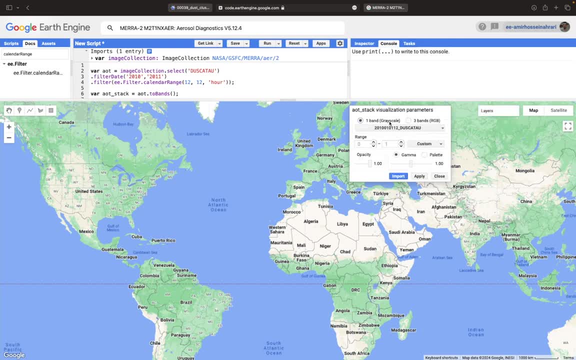 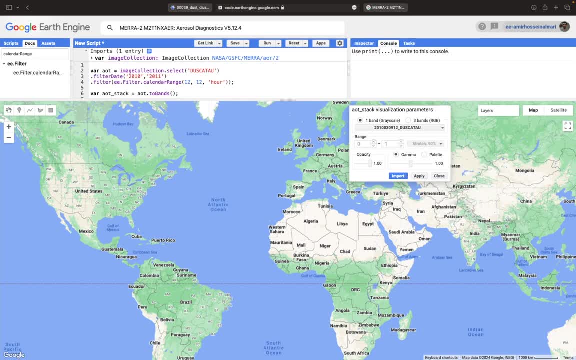 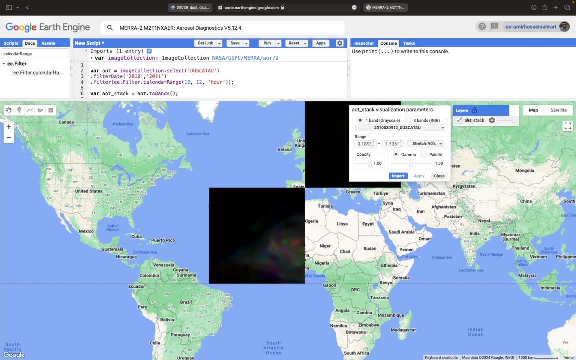 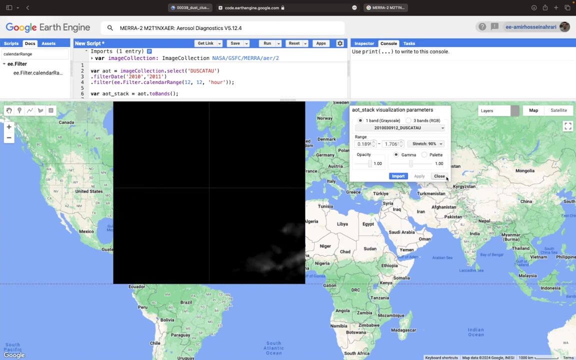 Select one of them and then, through the stretching technique, increase the contrast and once the contrast increased, you can tap on apply and then check it on for the visualization. I'm waiting to see the result, see the final map. so, as you can see, there is a gray scale image here that in 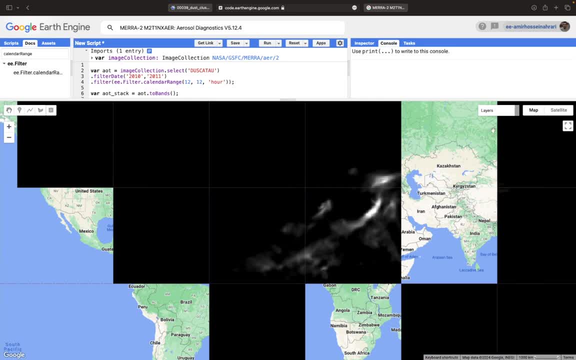 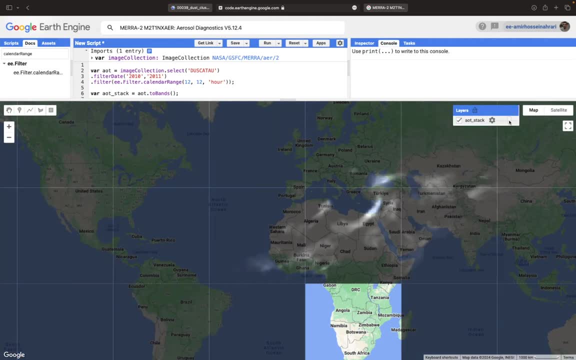 which the lower values and darker region shows the lower our soul or lower dust, lower dust and hazy condition, and higher values and brighter region showing the higher dust condition and higher dust storm or our soul in the air. so as you can see this region, that in this region with the brighter color and higher 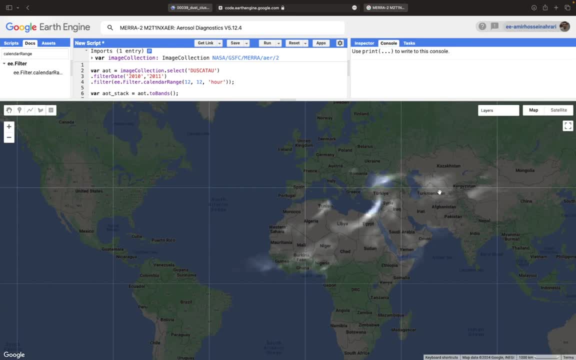 values definitely have higher dust or our result in this state and the rest of the world, compared to this region, are darker and they have a lower dust condition, so throw the inspector. if you click on the bright region, you can see that it has a. it has a. 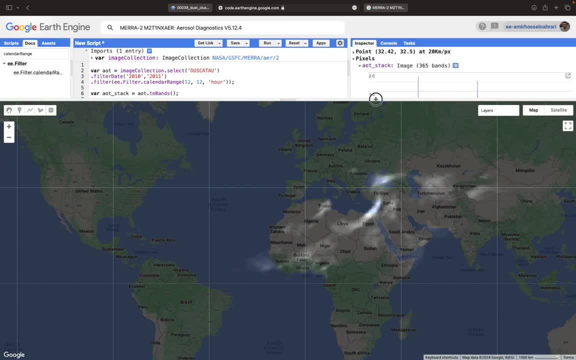 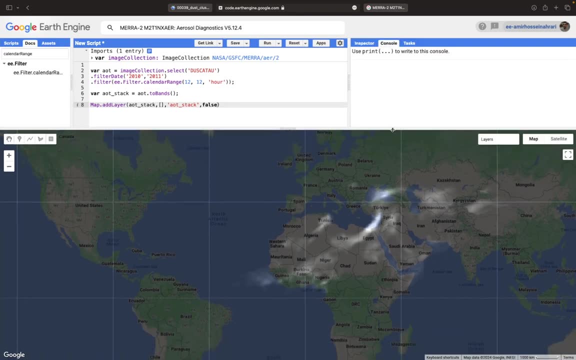 single value in each date, that each value plotted through the AOT stack. if you want to see the variations of AOT over the one year, it's very easy to select a point. throw a marker here, for example. throw a a marker. i'm gonna select a region in a libya, for example. i'm selecting a region here and then. 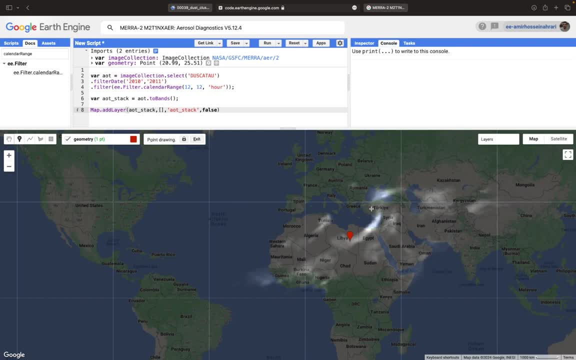 i want to monitor the dust condition or our cell in the air in the 2010 using a plot function. just use the user interface: chart imageseries helping you. using imageseries helping you to see the variation of the aot for the selected point. instead of image collection, you need to import. 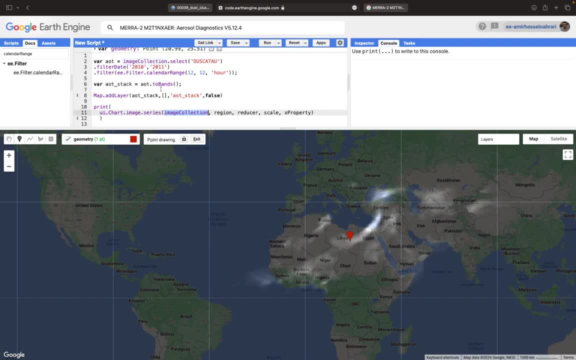 an image collection, not a stack. so we have aot here and instead of the region, the point or marker is geometry- already named here- and reducer. as we are working on a point, we need to plot the first value detected for the point earth engine dot. reducer dot. first, so, and then the scale. 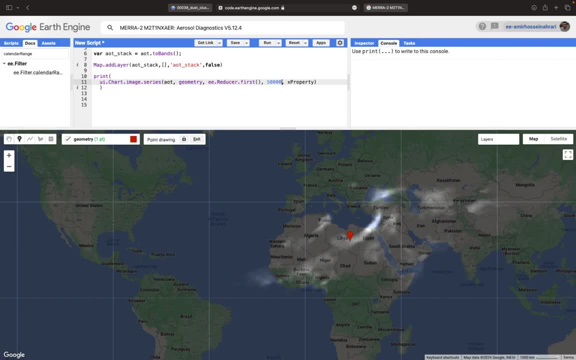 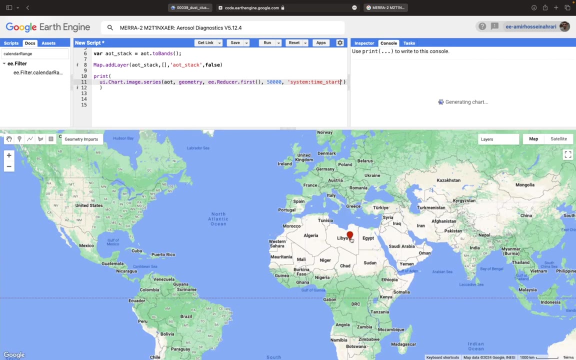 should be 50 000 because the spatial resolution is 50 kilometer and instead of its properties we need system time start, a main properties, a main property explaining the time information or date acquisition for the selected point. so again, after code runs, a new chart is generating. 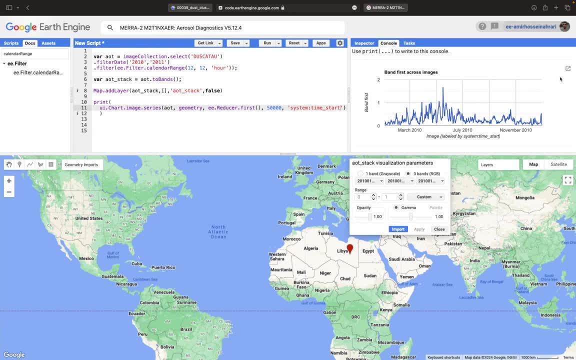 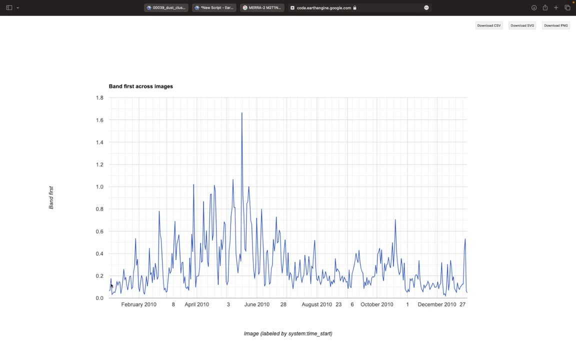 and, as you can see, the aot ranges from the zero between zero and two, and also when the aot increases from zero to larger or bigger number, meaning that the the larger amount of the aerosol or dust available exists, exists in the atmosphere, for example, when aot increases or 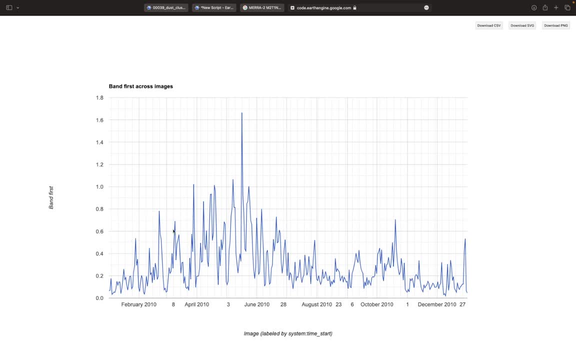 goes beyond the 0.5 or 0.6, meaning that this is not a simple aerosol in the atmosphere in such kind of condition, in higher and higher values, meaning that we have a dust storm or very dusty situation in that region. so you easily you can monitor the dust condition. 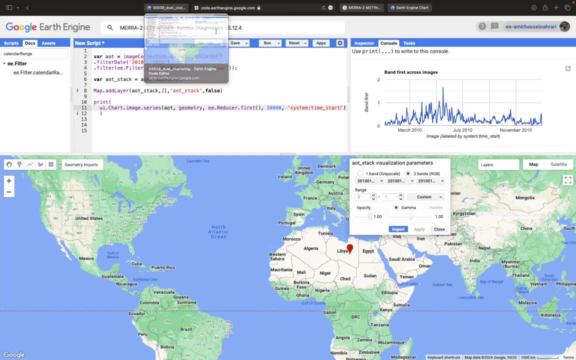 for a larger time scale or for a longer time scale in the google earth engine platform. here for a tutorial, i have selected only one year to show the results quickly. but you can extend the time scale to your own personal needs and you can also use the temporal uh temporal filter from. 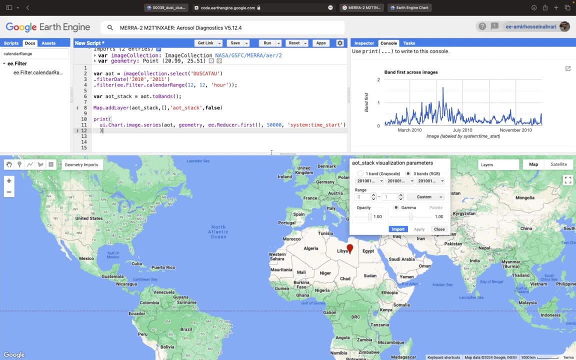 one year to 10 years or even 20 years to see the variations easily and accurately. in the next step, i need to compare the dust condition or aot values between two points. let me to do the visualization again, again, randomly select a date and or your target date and increase the count to a certain. 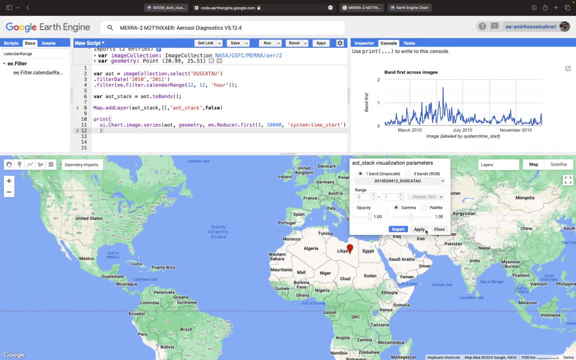 difference and the mayor of that event itself. according to that, of course, can hold two minutes for a player to tap the filter and click display tweeks under the seria icon. here i will decrease the tweeks for this particular event because the data inpa value is larger and 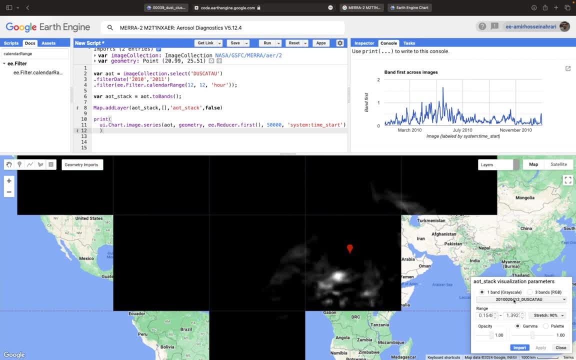 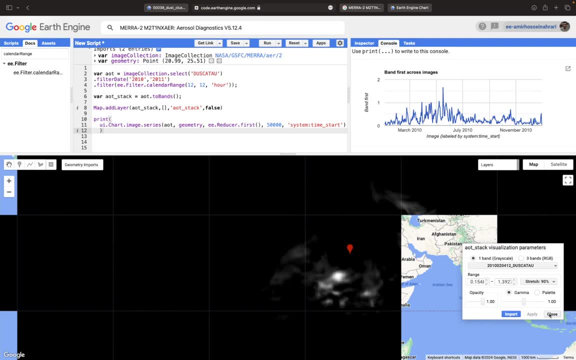 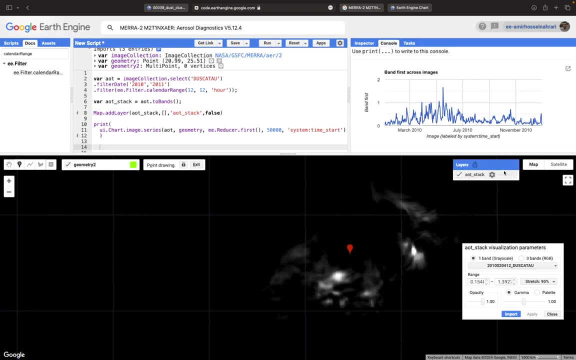 also, e inp is higher in price of this event. but for this case, this is my instincts for a very long period. a non- belongs to a really high amount of. I want to select another region, for example. I want to make a new geometry here, throw a new layer and here you can see the distribution of dust condition. 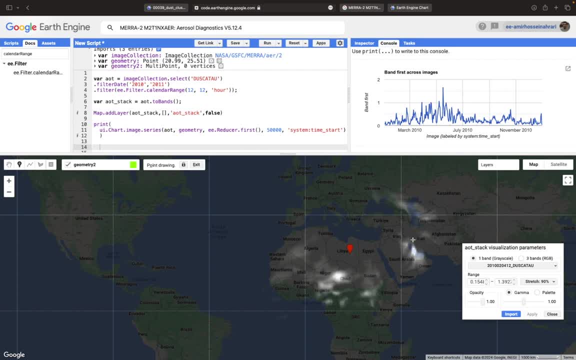 for these, for these states in all around the world. for example, this region in Iran is covered by the dust or our dense, our cell condition. so I want to select this point with a point in Algeria, to compare Algeria, to compare their a OT values in 2010: the first point in the desert in the central Iran and the second point 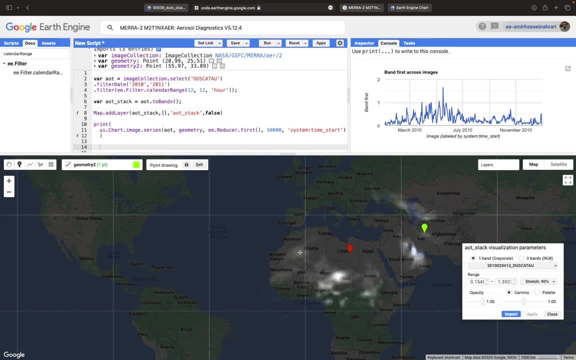 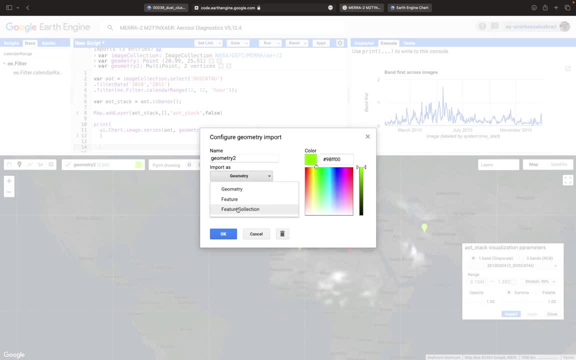 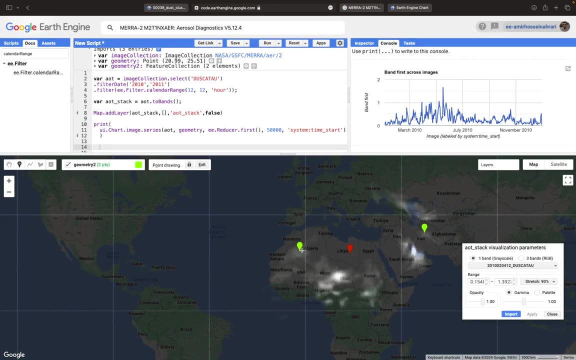 located in the north of Africa, in Algeria. so here, before doing further processing, we need to convert the geometry to a feature collection, because when you want to compare two points in the time series, you need to have a feature collection instead of a simple geometry to compare between two or multiple points. there is a simple 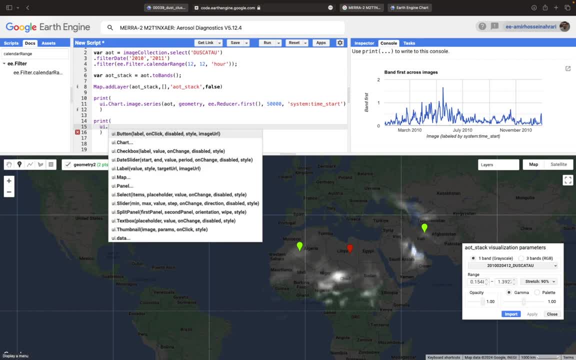 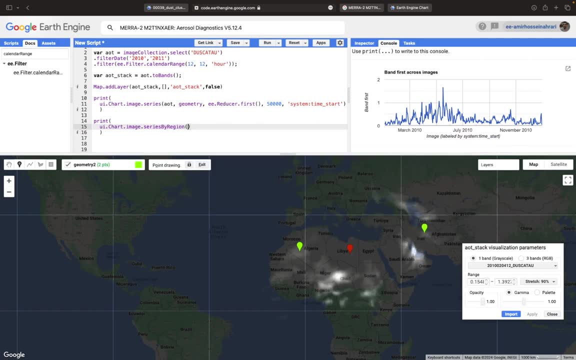 function in the time series and it is called a feature collection in the Google Earth engine platform. again, user interface chart image. but this time series by region is going to help us to visualize the changes, or plot the changes in each point separately and compare them into a single plot, the. 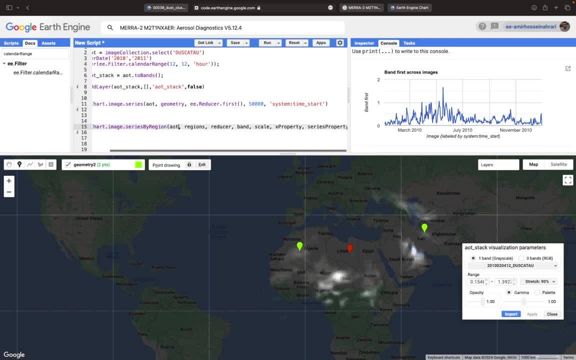 input collection will be a OT again and the region this time. instead of geometry we will have geometry number two, that it is not geometry anymore, it is a feature collection and for each point we want to see the reducer got first, the first value that's touched by point. so the band name, as we mentioned earlier, is this: and copy: 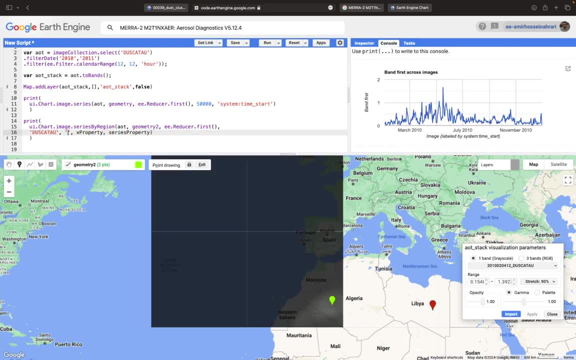 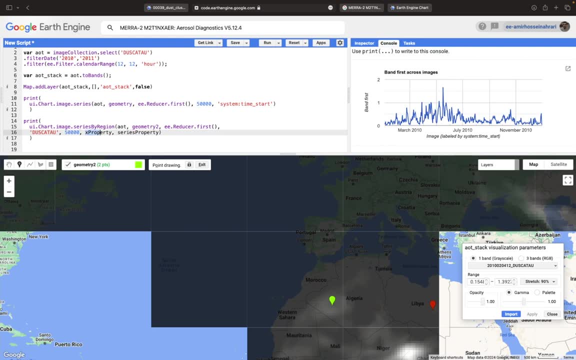 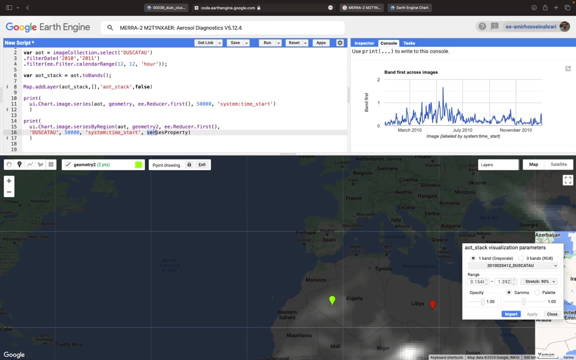 and paste of date name and instead of escape, you need to import the spatial resolution value, that is 50,000, and instead of x properties, system time starts like this: and instead of series properties, the series properties referring to that column. that's separating the 0.1 and 0.2. 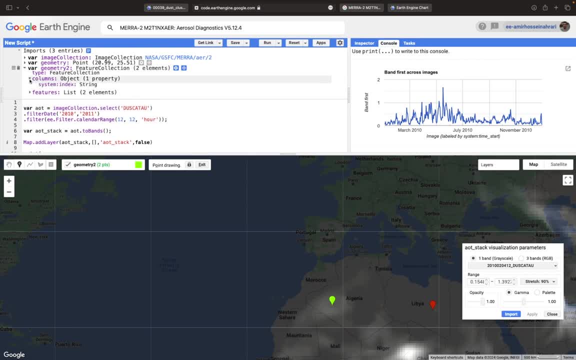 if you go to the geometry structure you will see there is system index for all shape files imported into the earth engine, or all the feature collections you make. here you will have a system index that helping you, separating all features by a single number. so now here, import the system. 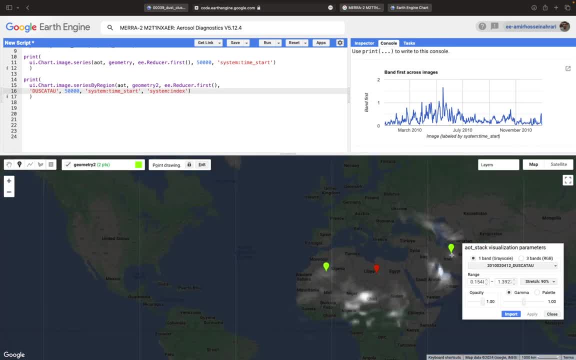 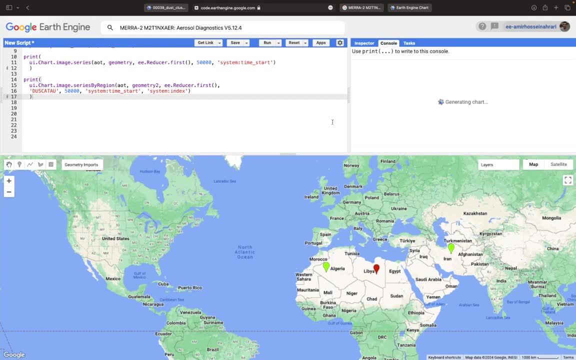 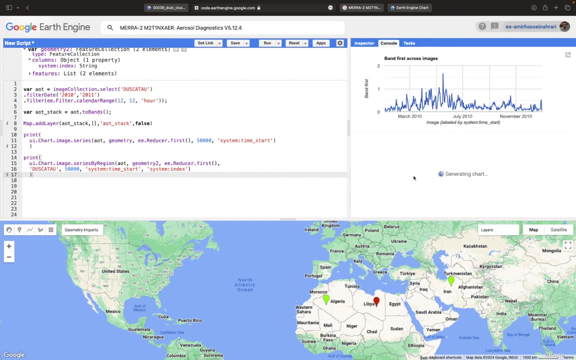 index, the index number 0 is the first place and the index number 1 is the second place. so and then run the code and after a few moments, in the new chart you will see the variation of the aot between the first and second place, the first point located in iran central desert and the second point located in the 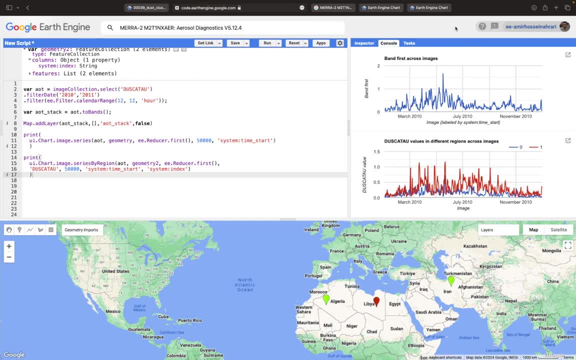 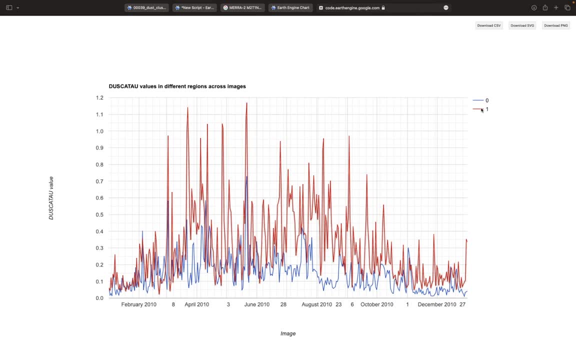 north of africa, algeria. so if you go to the more details, you will see that obviously the red region, the north of africa, experiencing higher dust condition, uh, compared to the central iran, and also if you see the pattern of dust changes or aot changes, you will see that. 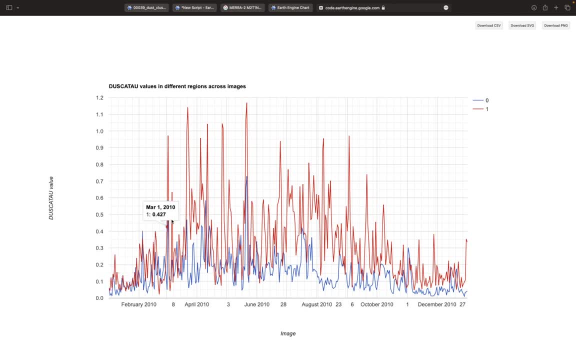 there is an increasing trend from the starting year, from the start of year to the summer, and then the creator is a decreasing trend toward the end of the year, meaning that in the summer time or drier time during a year because of low precipitation and low moisture content in the region of interest, we will have more aot or our cell or dust storms in. 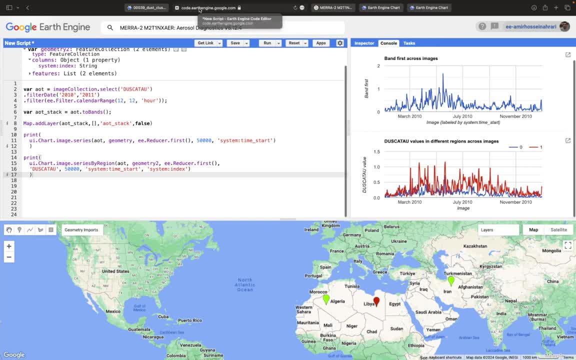 that region. that makes sense. so back to the programming step. in the next part i'm gonna show you how to do the time series clustering, how to do how to make a clustering map for the dust condition to separate the regions according to the aot condition. now, in this step, we want to cluster all, all the regions based on the 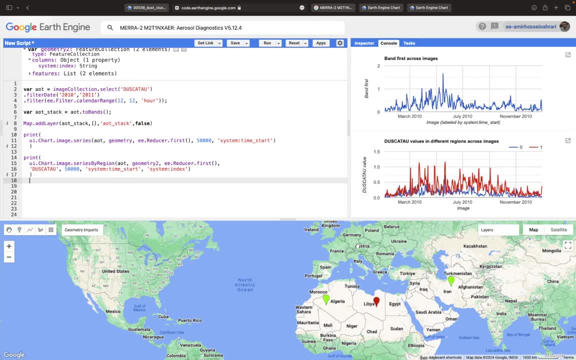 characteristic based on the characteristic distribution and the values of aot. so here just i'm making a a new session about the clustering. this is the first time in this tutorial in my youtube channel i'm talking about the clustering technique, or unsupervised classification. clustering, or, 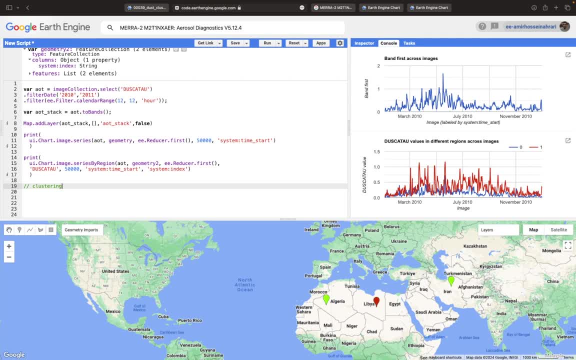 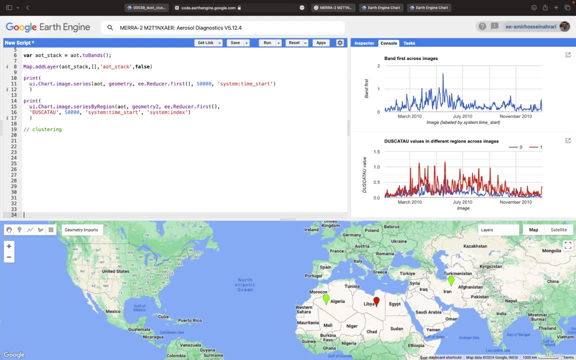 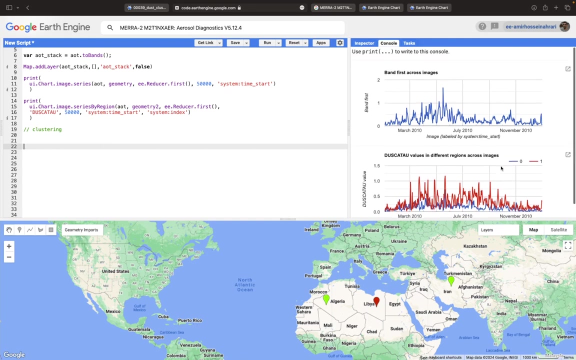 unsupervised classification is a kind of learning method in the machine learnings, that available in the remote sensing, that helping us to categorize our data without uh categorize our data automatically, also without doing sampling by the user. so for example, here i have 365 aot values and i want to 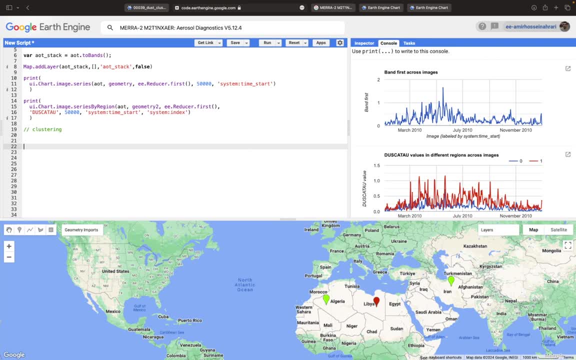 classify all the region of the world- or all the regions are under study- according to the value changing in this product. so first we need to collect some samples automatically in the clustering method. you don't need to do a sampling process by the user, that all the process is automatically. 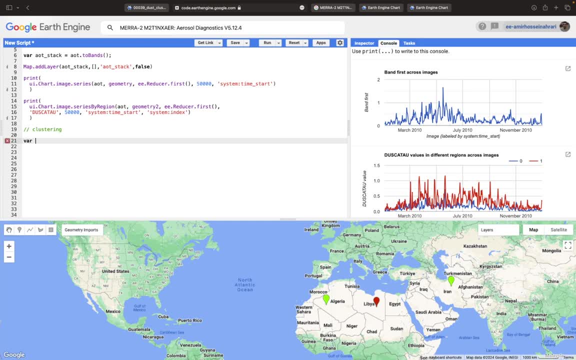 and also even sampling parts make a new variable. for example, this is samples equals to from aot bands or aot stack layer. i want to collect the samples. there are some arguments that should be considered in the sampling process. the first is the region of interest, the region in which stamp we want to. 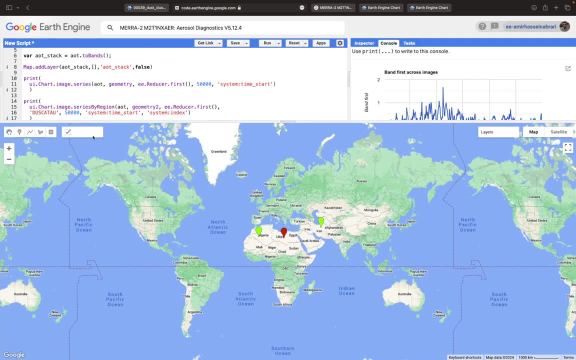 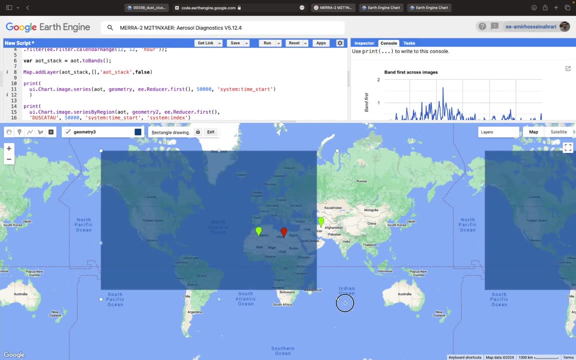 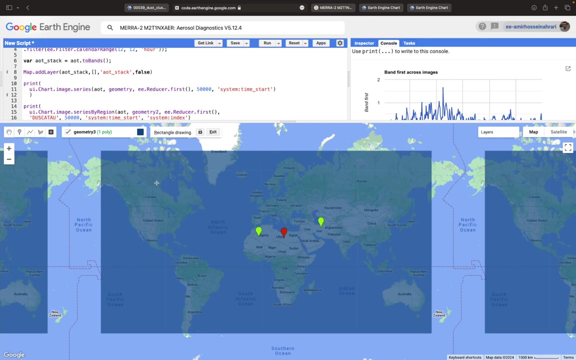 do the sampling so, for example, i can select a region through a geometry, imports in global scale, for example, i'm selecting whole of the world, like this and, as you can see, hold the board selected in this study because i want to do the clustering, i want to collect the sample. 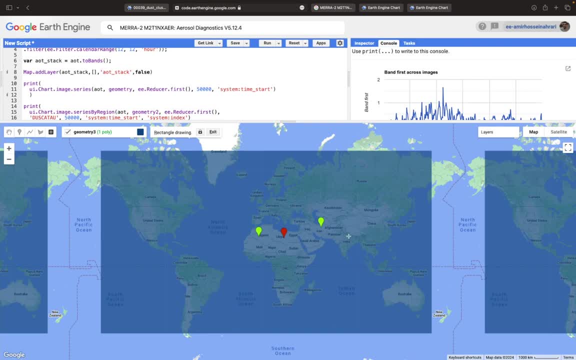 according to this region specifically, and also it's very important that your geometry covers the dry regions. in their uh, in their, for example, dust condition, mostly occur during the year or during uh days. so, as you can see, the region now is equals to the geometry. number three and another important 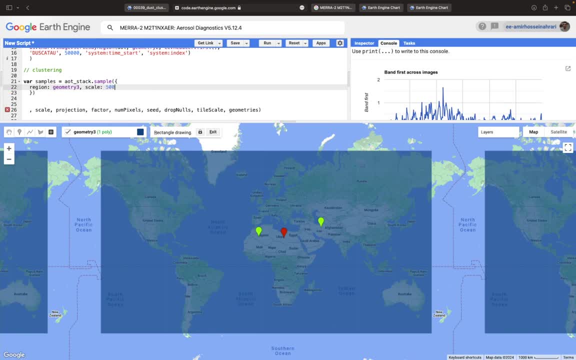 argument is: scale equals to 50 thousand meter and the number of pixels that we need to collect as sample equals to, for example, 5 000 or even 10 thousands. as we are working on global scale, you can select a large number of pixels for the clustering. so, after samples collected using this method in the next part, 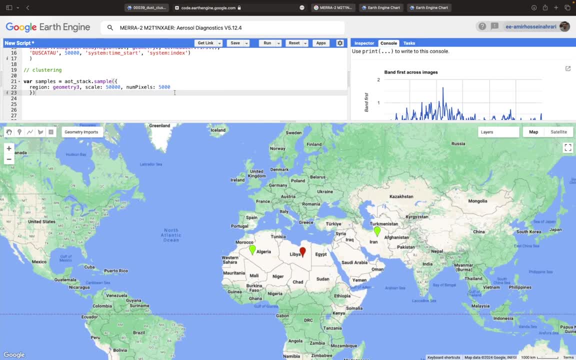 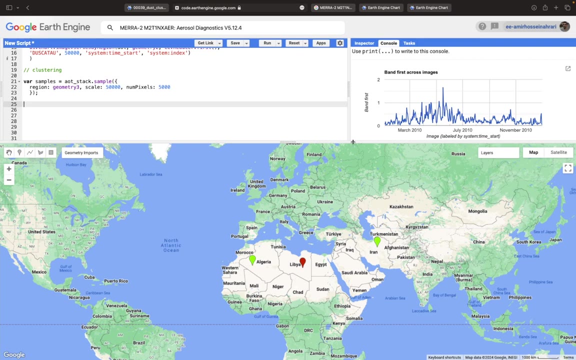 i'm going to. i'm going to define a clusterer here using a built-in function in the Google Earth Engine platform. One benefit and advantage of Google Earth Engine for users is that the various functions for the machine learning analysis available there and for the users using the built-in structure and you don't need to write very complicated. 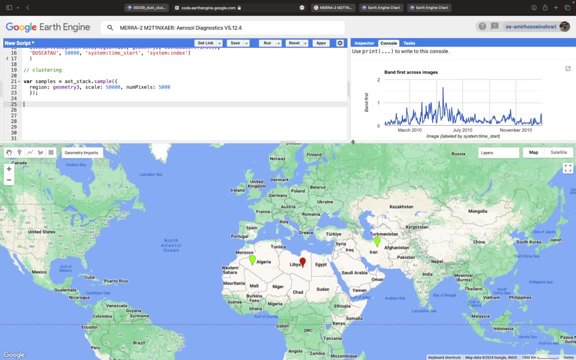 or tweaky code to do a time series or to do a mapping process using machine learning algorithm, and also this is the simplest way for the automatic clustering method that I'm showing you in this process in this tutorial. So in the next part now I'm making a clusterer, for example. there are various clustering. 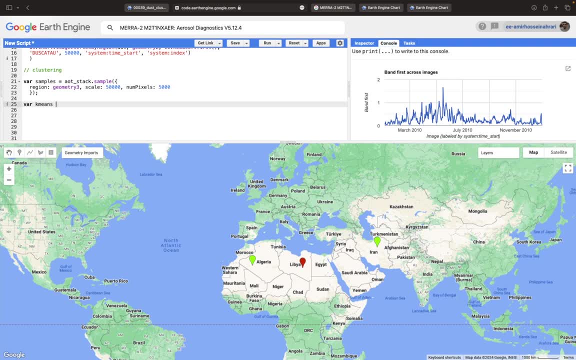 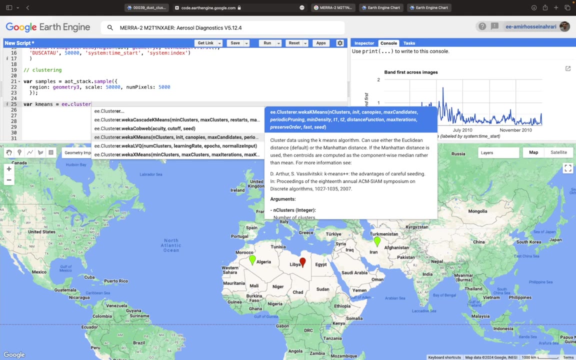 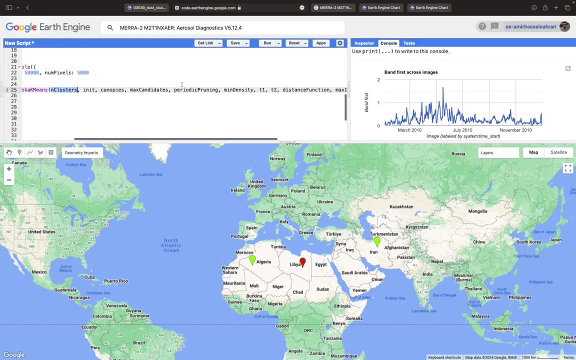 technique in Earth Engine, but one of the most famous ones in machine learning is K-means And here through the Earth Engine dot clustering or clusterer, you will see that how many clusters available here, for example, I'm going to use VECA K-means here, The VECA K-means. multiple arguments available, but most of them are. 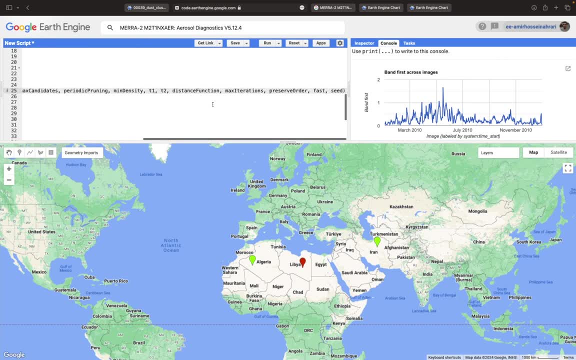 optional except number of clusters. It's very important to set them. it's very important to set the number of clusters before first further steps. For example, I want to classify the AOT in all around the world into five or four classes because I want to cluster different regions or see the 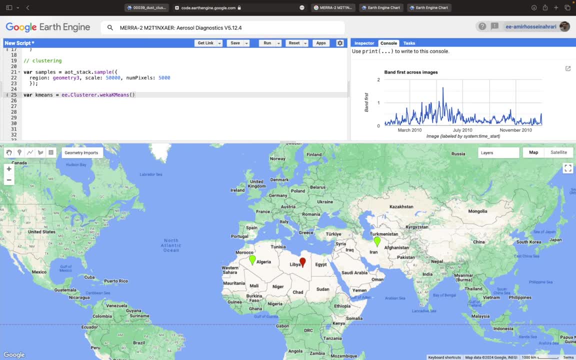 different clusters according to the density, according to the density and also the stability of the dust or AOT, using clustering technique. So, For example, I sleight of hand enough for every cluster in the timeline I'm setting number five as the number of clusters, and then I want to train this. 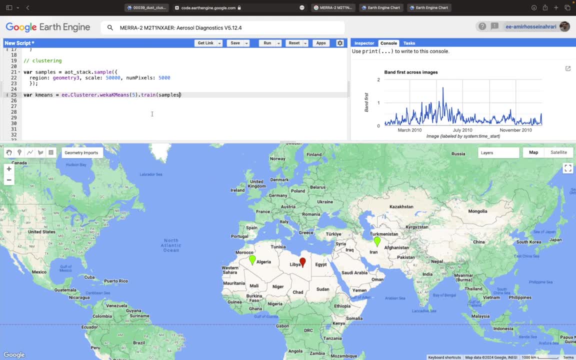 model according to the samples collected. So K-means helping us to make five Clusters according to the samples collected from the AOT's stack. So in the next step, K-means module helping us to cluster all AOT orders- training cluster. I see. 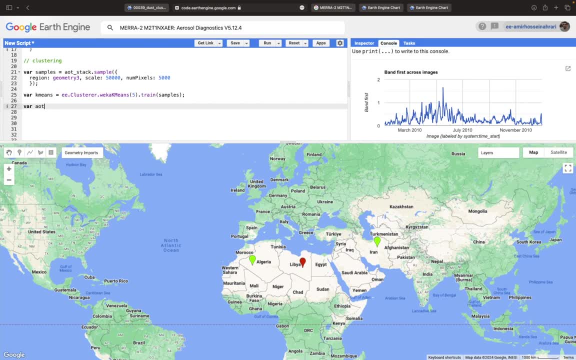 stack file. Here we have an AOT map. equals to AOT stack imported into the model using clustering function, dot cluster based on k-means. I'm going to cluster AOT stack according to the k-means that is already trained, based on the number of pixels collected from AOT stack in our region of interest and 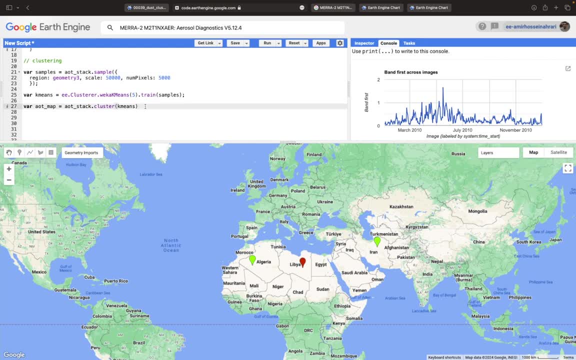 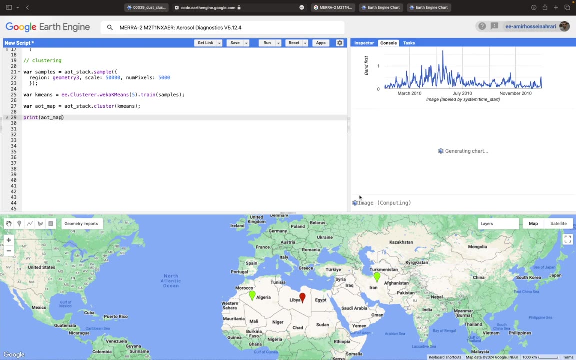 according to the scale or spatial resolution. So finally, I'm gonna print AOT map to see if there is any syntax error or not. In the right panel, one image is under computing because we will have one clustered map. It is under computing and once the process of computing is over we can show the result and visualize it in. 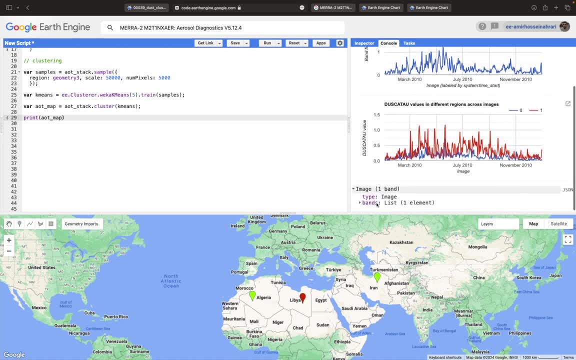 the earth engine. So image with one band makes sense and also meaning that there is no syntax error in the clustering techniques, because we not faced with any type of errors in this regard. Then, through the mapadd layer, you will be able to see the AOT map. 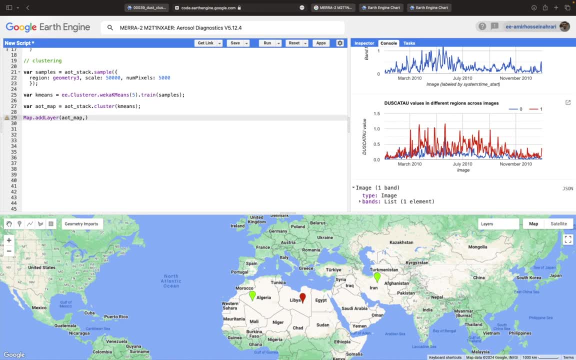 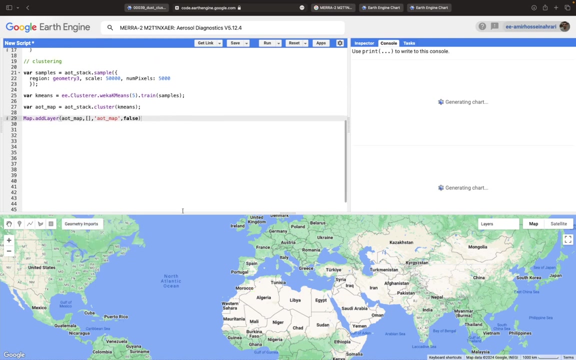 or clustered map and no need to clip it based on the region, because I want to see the clustered map in the global scale and leave the visualization empty for now and then. the layer name is AOT map and use the false to avoid automatic visualization process. Check out the geometry imports and here, through a layer, you can see the AOT map. 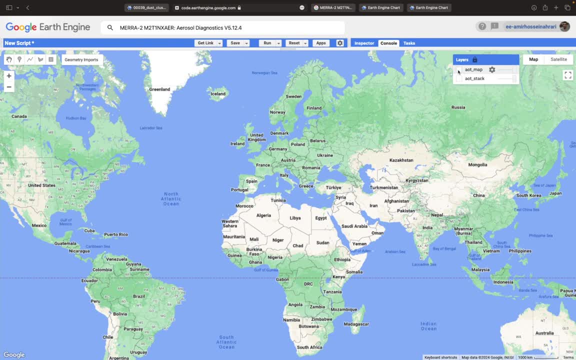 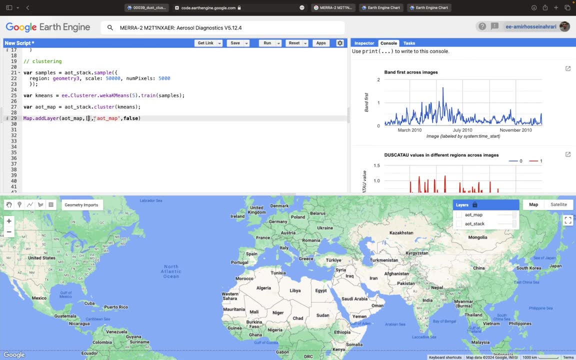 You can click on the AOT map to show the result to to have a better visualization. As we have five classes, it is anticipated we have five number of classes, from 0 to 4. so here to better visualization, set the min equals dough means as equal equals. 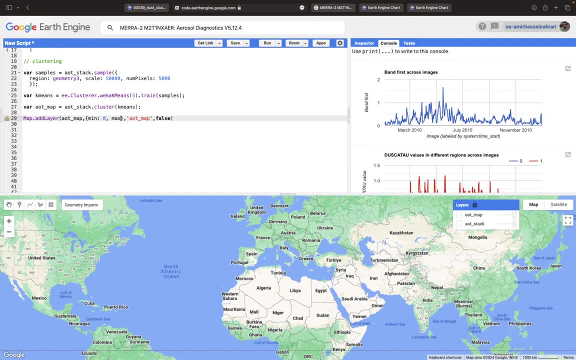 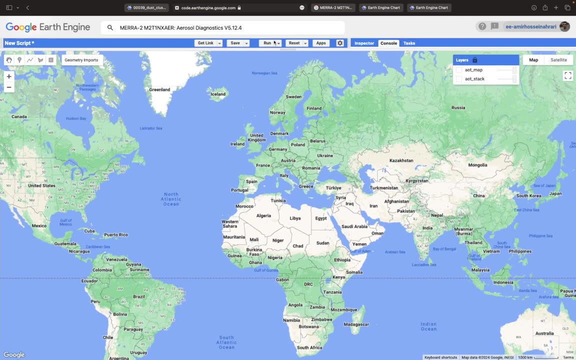 mean 20 and then for the max, set it number 4 to avoid any enhancement process. so run the code again and click on a OT map. now I'm waiting to see the final result. that is clustered map. clustered map according to the: a OT characteristic in 2010. this is a. 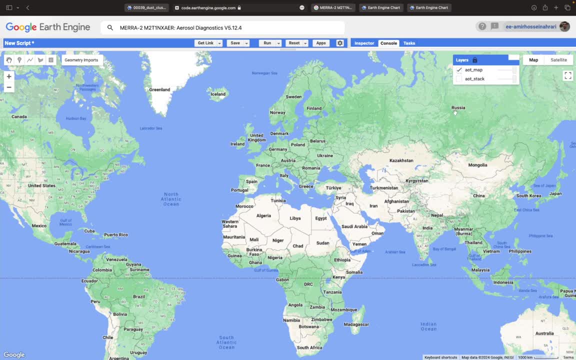 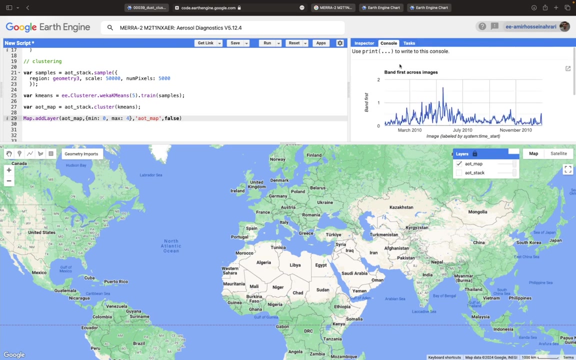 clustering map only for one year. as we use the large number of images for the clustering technique maybe it's a little time-consuming process to see the final results. but be patient and also wait to see the results. if there is any problem happens in the processing and also it will be showed in the console part. so 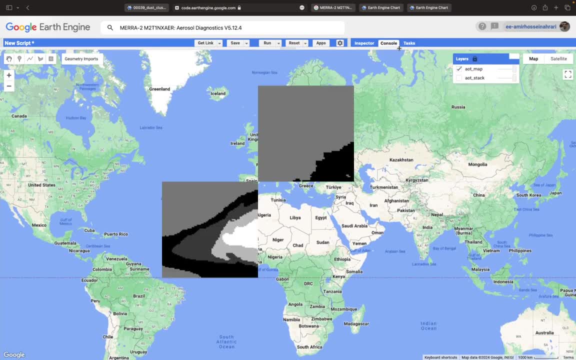 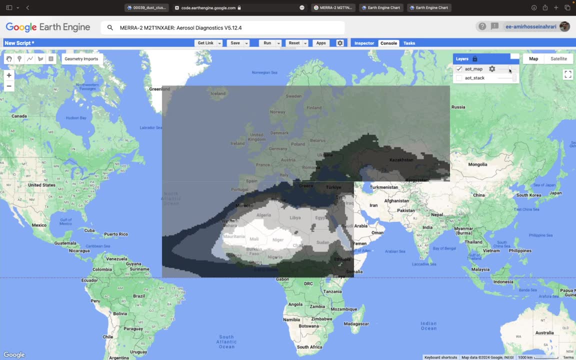 still, we are waiting to see the results, see the final results. as you can see, the final map is created, a final map is created for all around the world and you can see that the different regions classified based on the, based on the condition, based on the dust condition. 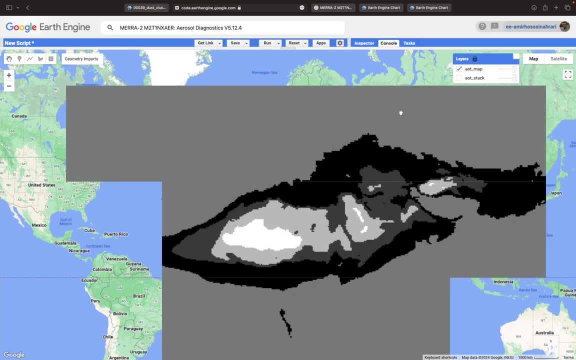 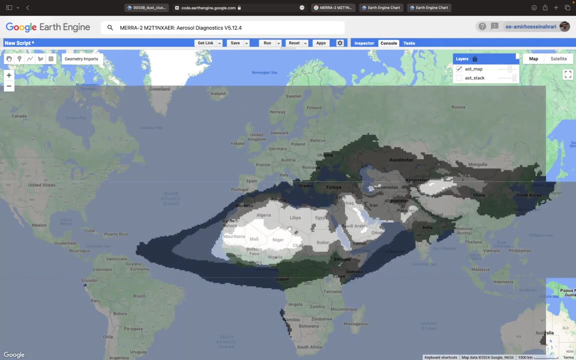 for example, here we have a 4 class, we have a 5 class map. for example, that, with only a bit variations, only in the mid-latitude regions or in the places that mostly covered by the, by the actually deserts, or these are mostly covered by the drop dry regions actually, 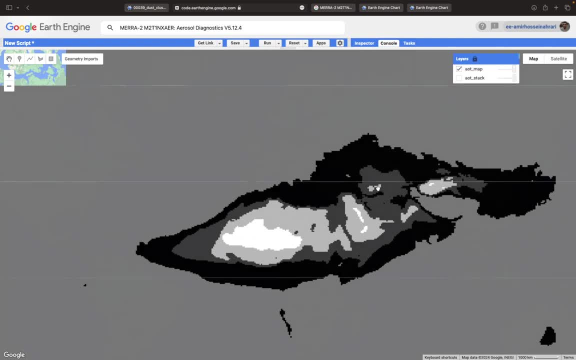 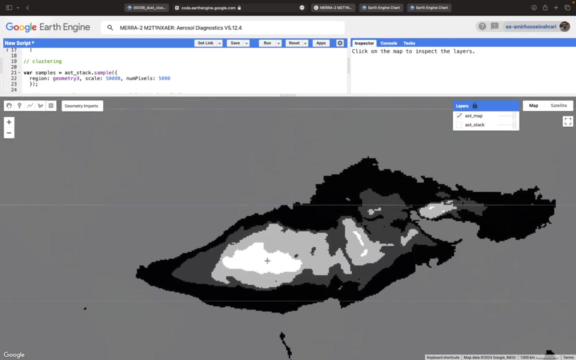 so and then you will see that this is a very, very clear map that showing the variations of the dust in this region. so, in order to have a better visualization, through a palette you can increase the contrast, you can increase the quality of map by setting a palette or color. throw a inspector if I click on this region for. 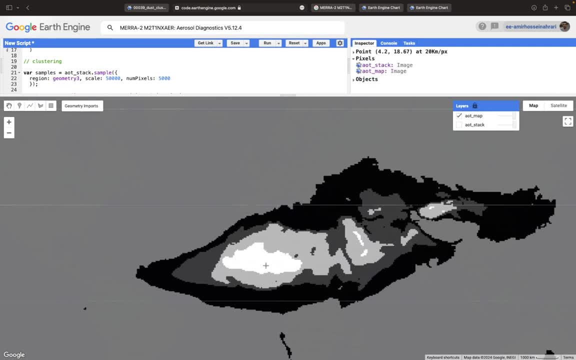 example, these regions value. I need to know that. which value showing this region, cluster number four. so the last cluster is number four and the next one is the next class value, for example, is number three. yes, and now we can set a palette to visualize better. for example here: go to the pallets, go to a palette and 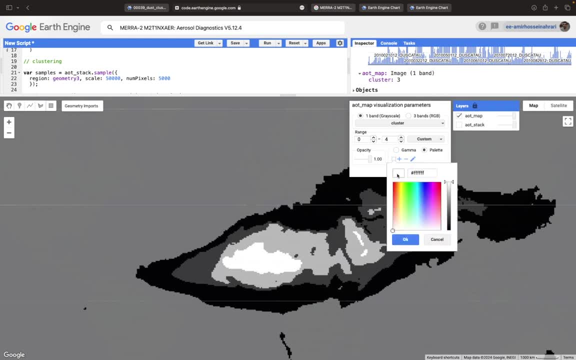 define the colors. so the first, the first class value- I assume that's the first last value- have the lowest cloudy condition, for example. here I set the black color for this region or no, for example, blue, yes, and also I'm setting colors manually without any standard, but you can set a standard color for the final map. 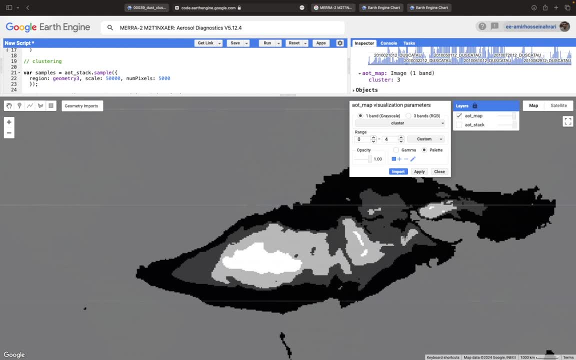 just, I want to show how to set the color and how to visualize it, and I'm not following any specific, any, any single standard for the coloring, the dust for the coloring, or to set a palette for this map here, for example. then I have green, then the yellow and then orange and finally, 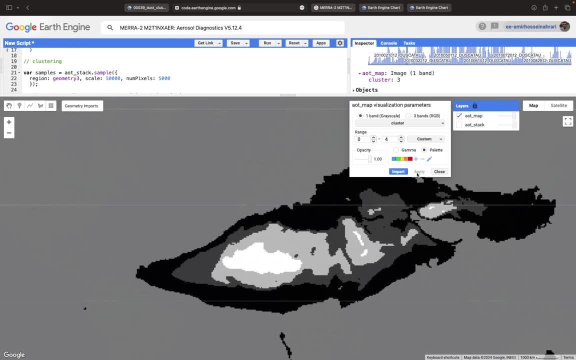 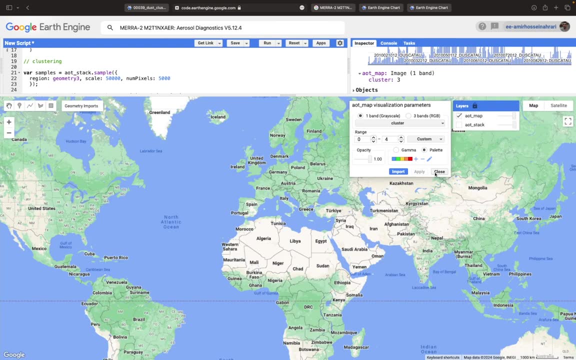 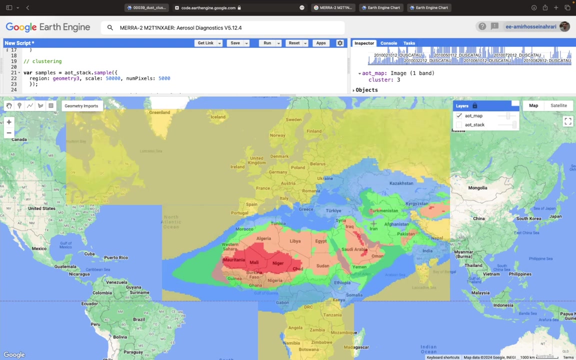 for example, I have red here, so apply it and then you will have multi-color map, you different classes available here. the map is creating, the map is creating and also you can change the color, you can change the transparency to see that which countries are which, which countries included in which classes, for example, North of Africa, that. 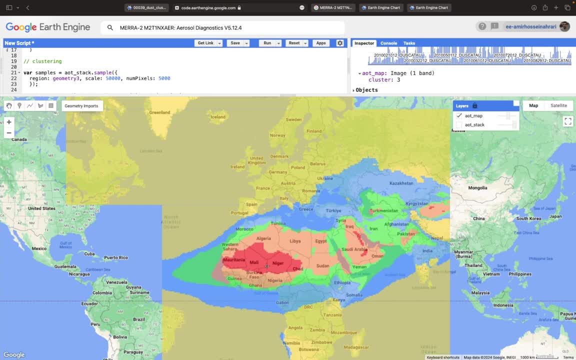 is the most populous country in the world and you can see that the countries that are in the is one of the main centers for the dust events or something like that. North Africa and a part of Middle East colored by red color and these region, meaning that this region, have the same. 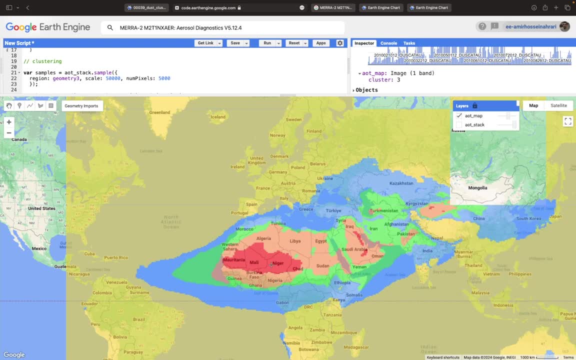 characteristics regarding to the AOT values and changes and the next class, that here and the next class with the, for example, lighter red color. you can see here the next class in Egypt, Libya, Algeria, showing that having shows that they have the same a OT characteristic with Saudi. 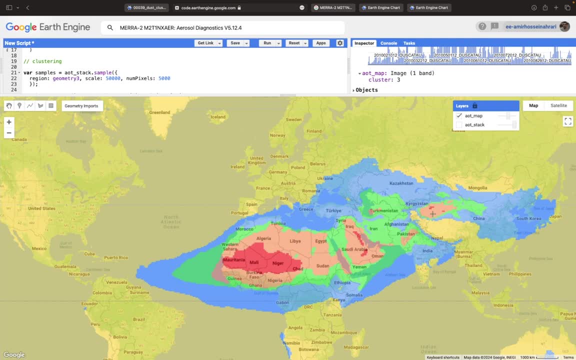 Arabia or this region in the China. so that's this kind of maps helping us to compare different regions, to understand the similarity or differences, for example, in a global scale. there is no dust event in there. for example, European countries and also Eastern countries, your Eastern European countries, and also. 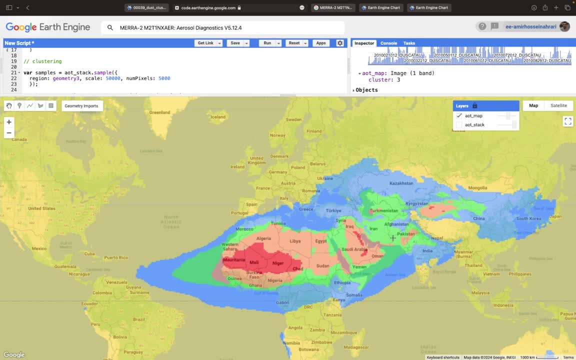 western countries, at least compared to the main, compared to the, these dry regions or this, yeah, Africa country is the African countries, then the number of events or the number of dust situation is really, really low and is and also is ignorable in our map, because the most of dust events happening in this region 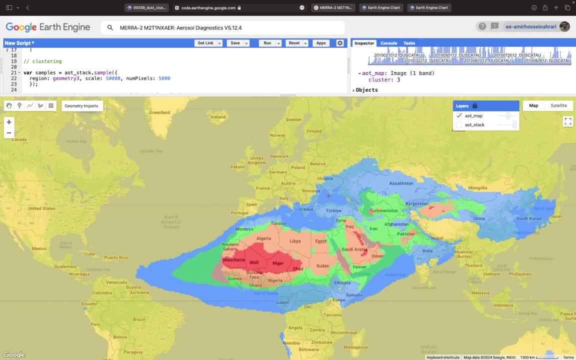 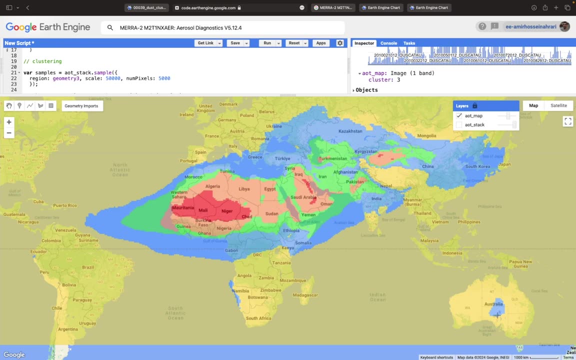 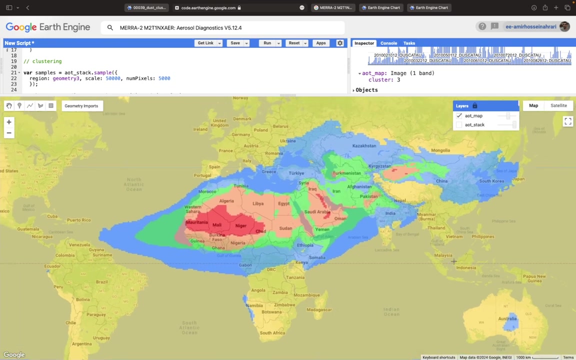 according to the classification, we have done so. or even if you go to the house- uh, australia- you will have some anomalies in the center of australia, meaning that sometimes some dust events happening here or uh. or, for example, regarding to the aot, you will see that in iran. 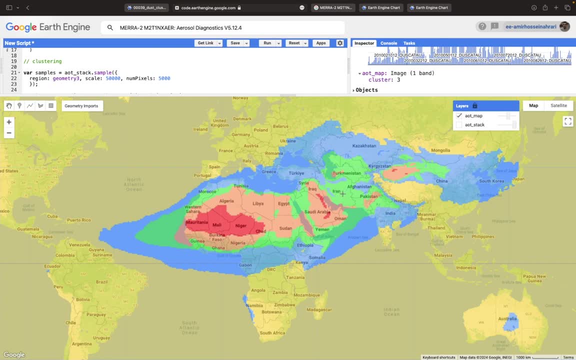 uh, there is in the central part of iran. there is a similar characteristic with, for example, the other countries in the uh, africa in the north, in the egypt, in a part of egypt, in the part of saudi arabia, in the yemen- they have same aot characteristic- or with turkey. 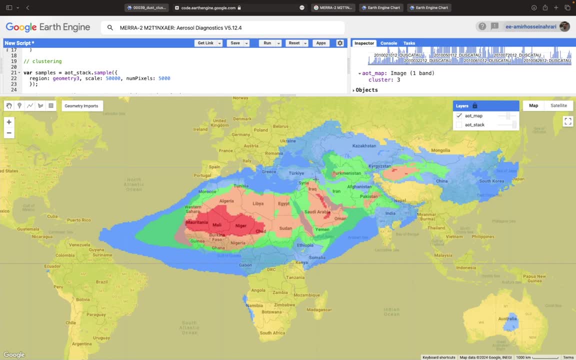 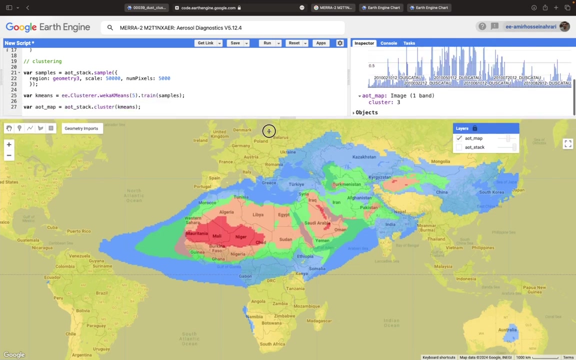 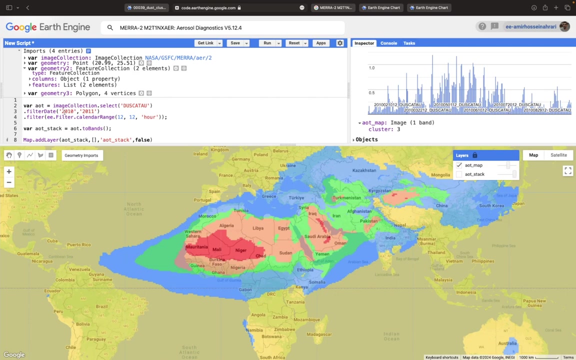 minister, and also, yes, this kind of map helping you to understand the, to understand the dust situation and aoc similarity and differences in all around the world, that is very, very useful to understand and to understand and interpret the dust situation in different countries. you can do this. you can do this clustering method for a larger time scale, extend, or even you can. 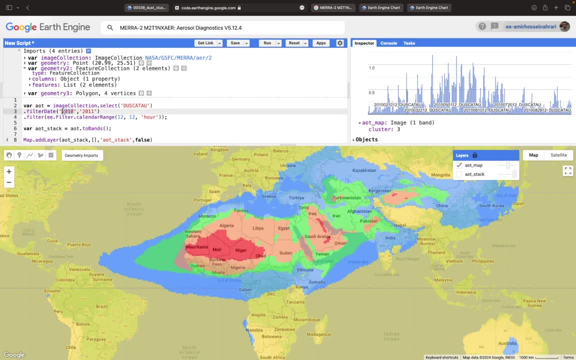 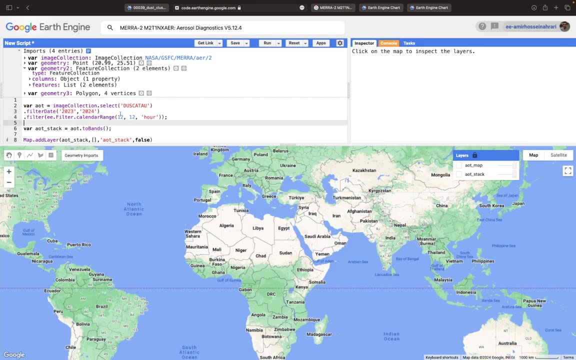 use it for, for example, the another year if you want. for example, i can apply this classification instead of 2010 for 2023, for example. we will have a new map only for this year, but in unsupervised classification or clustering technique, you should know that the class values may be changes from. 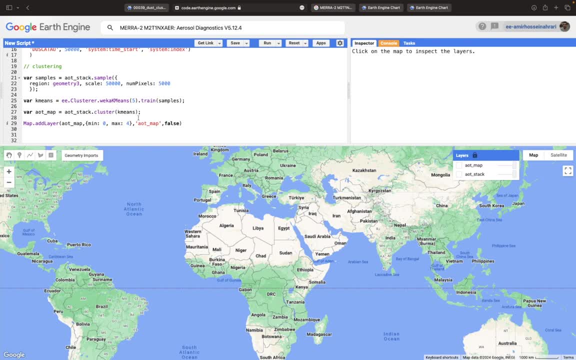 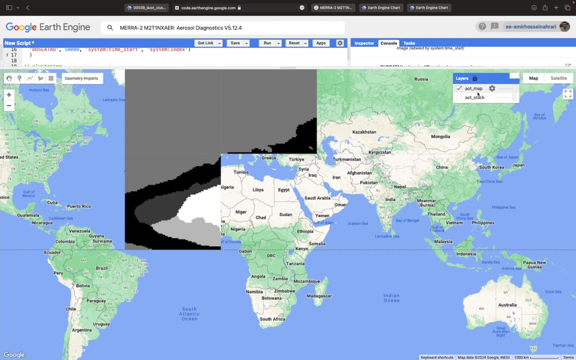 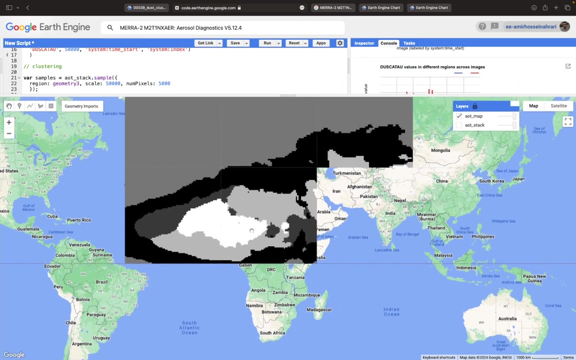 one date from one date to another date. for example, if north of, for example, in the previous map, the north of africa had the number four and identified through the class number four, but this time, uh, maybe we will have another value for the north africa. so check it on aot map again. you will have a new map and a new map with a new pattern. it's very 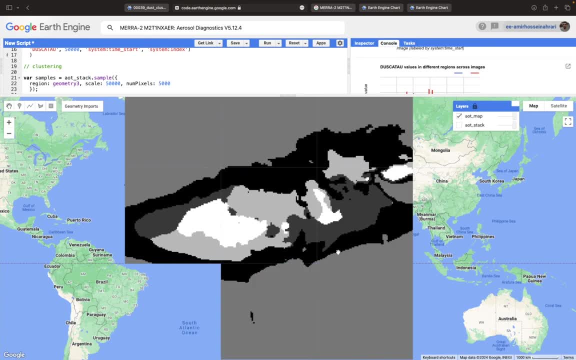 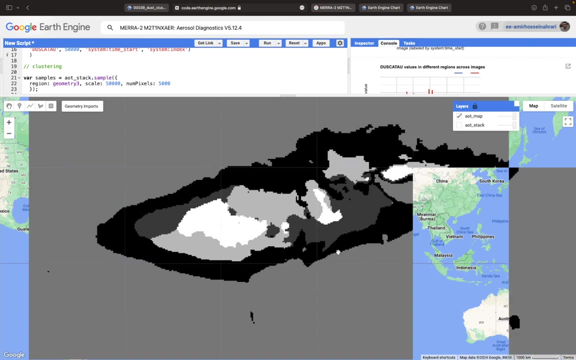 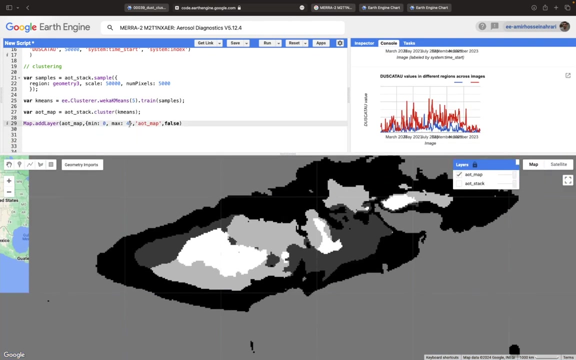 important because the world is dynamic and also from one year to another year the dust pattern may be changed and also it's very, very visible and makes sense when you see the changes in the dust patterns from one year to another year. again, throw a palette in the code. you can add visualization parameters. 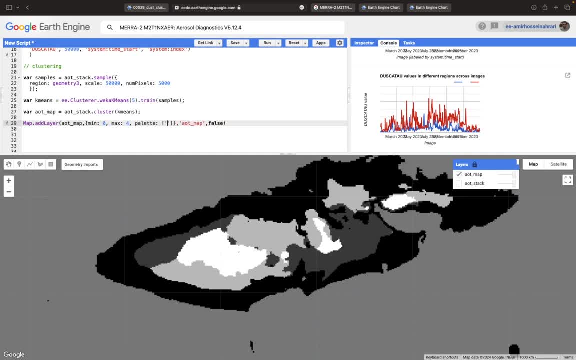 or call it, or color palette, to see the outputs more realistic. for example, i'm starting from white, you can set any color you want, but i highly suggest you to use the standard visualization uh for the visual, uh, standard colors for the visualization, to improve the inter, the. 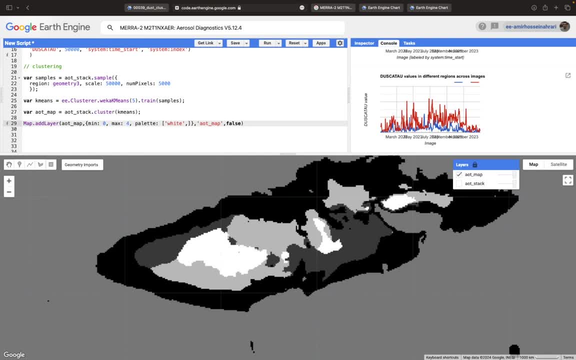 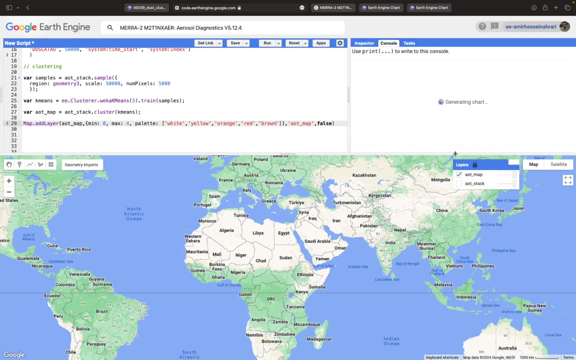 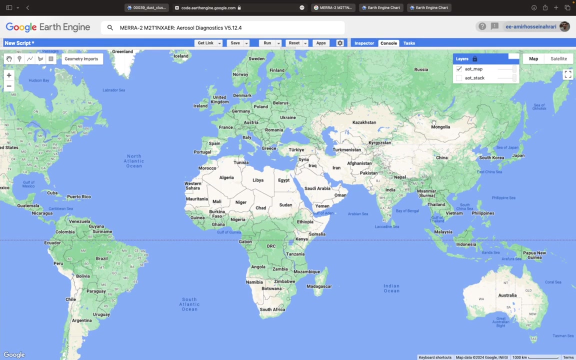 power of interpretation in your results- white, yellow and orange, red and brown, for example. click on aot map again. after a few moments you will see the new map that is created. if you had any problem regarding to the programming technique, the code, the code. the code i'm using is: 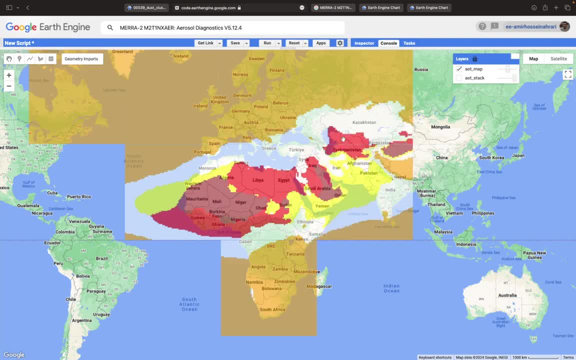 available in the description part in my youtube channel below this video and you can use it to compare it with your own code. and if a problem still exists, you can reach me out through my email address and i will try to help you to solve the result, as you can see, uh in the regions. uh, in the hottest hot spot regions. 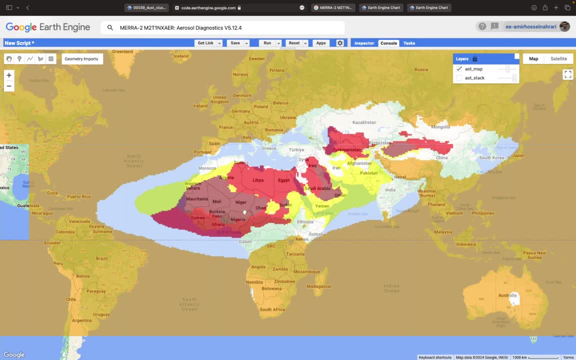 colored by a brown color in the north of africa, in the saudi arabia and iraq and also in the part of china, and then you can see the other regions with different colors. that helping you to understand more, and about the dust situation and similarity and differences. 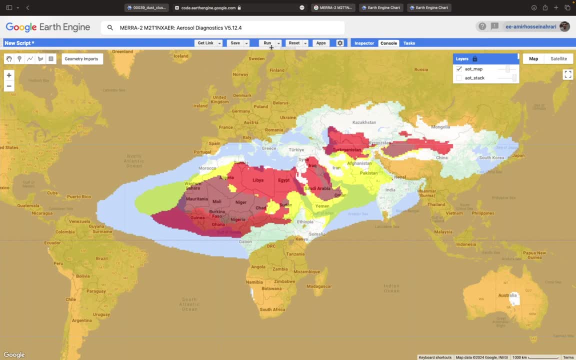 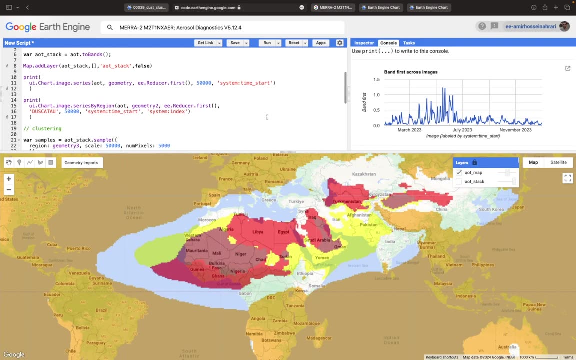 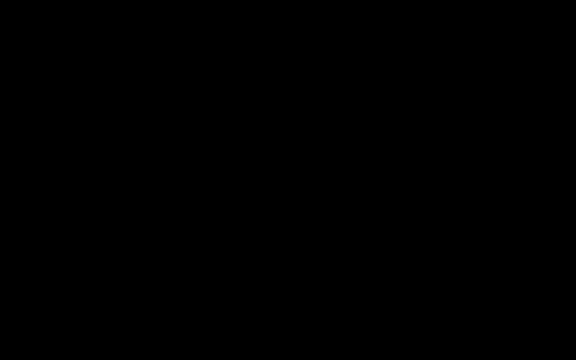 of different places. hope you like this tutorial as much as i did and also, if you had any problem, you can reach me out through my youtube channel. thank you for your attention.